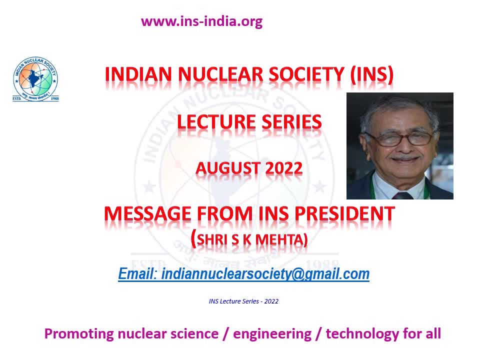 undergraduate students and general public knowledgeable in their respective fields of nuclear science and engineering For the benefit of the public. some of the important and the common application of nuclear being for power, industrial use, medical diagnosis and treatment, agriculture, food preservation and various. 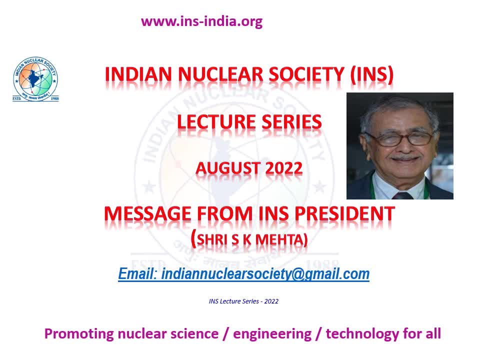 other areas. This lecture series is made in simple language and illustration with the aim to inform the general viewer about the science, engineering and technology that is involved in the development of nuclear science and engineering. Social benefits of the nuclear. application of nuclear carrier, benefits in nuclear and. 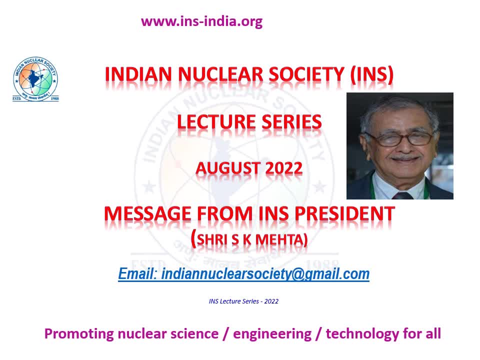 regulatory and safety of the nuclear energy. The presentations are prepared and narrated by experts on each topic in a way that the viewers with no background knowledge about the nuclear science and engineering can understand. Our effort will be to constantly provide information about newer benefits to the society emerging. 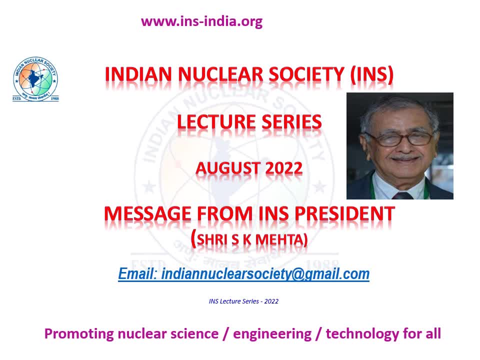 out of the pain-taking research and nuclear science and engineers. Viewers are encouraged to comment, suggest and put forward questions to the experts. The channel of constructive communication will always be open to discussion. Thank you for watching the lecture series by Indian Nuclear Society. there are 13 lectures. 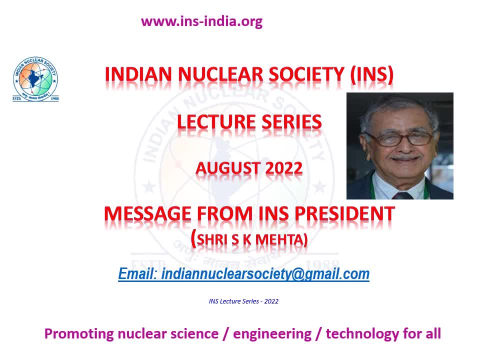 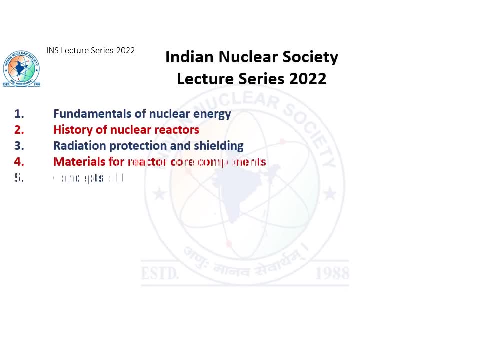 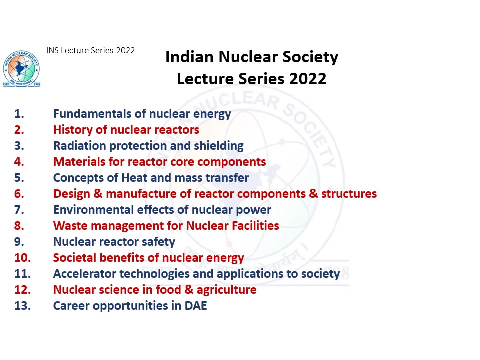 on various topics related to nuclear energy and its application to societal benefits. All these lectures will cover different aspects of nuclear science and engineering, as well as different topics related to nuclear energy and its application to societal benefits. Thank you. The lecture series will cover different aspects of nuclear energy in sectors like power medicine. 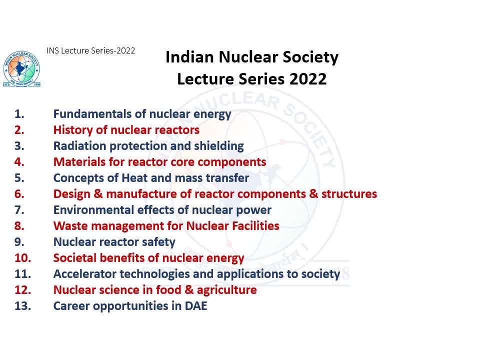 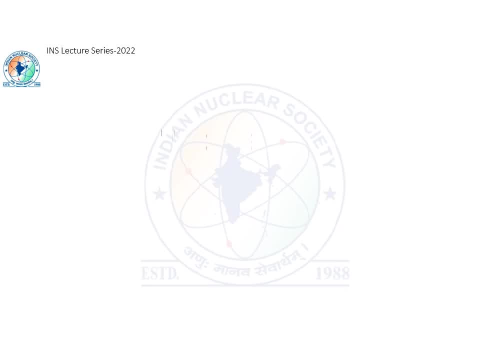 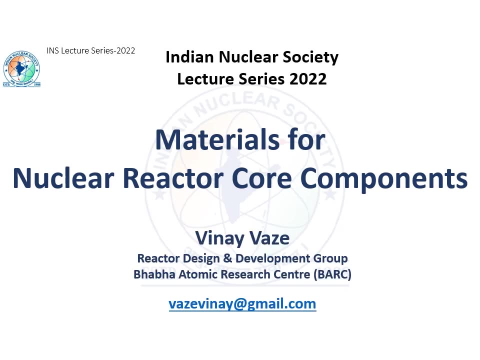 agriculture and society. It illustrates in simple way the science behind nuclear reactors for all of us. Hello all and welcome for this lecture from Indian Nuclear Society. Today we will discuss about various aspects of materials for nuclear reactor core components. This has specific focus on Indian Nuclear Reactor System that is Pressurized Heavy Water. 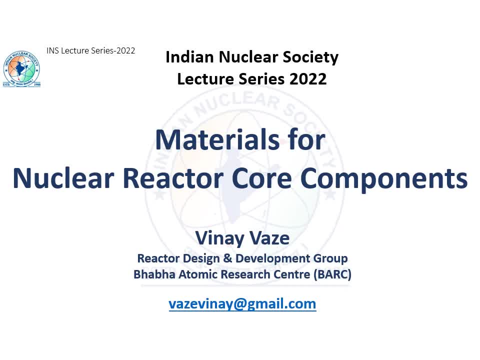 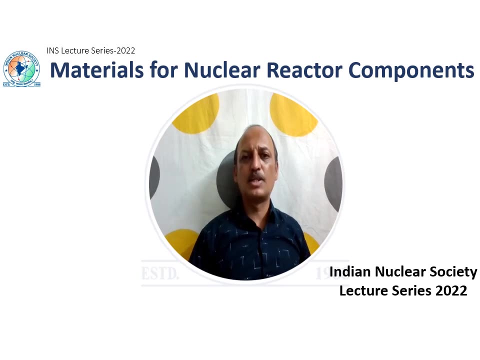 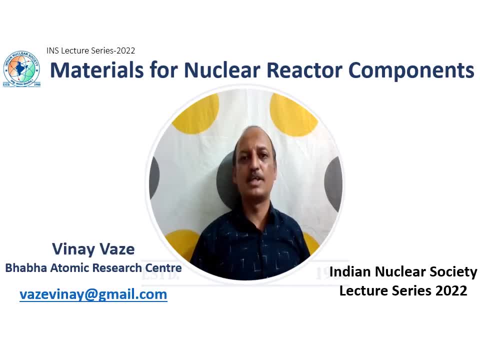 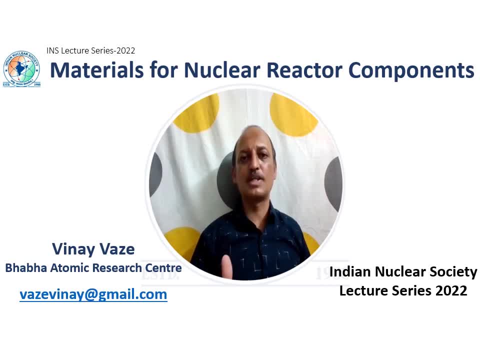 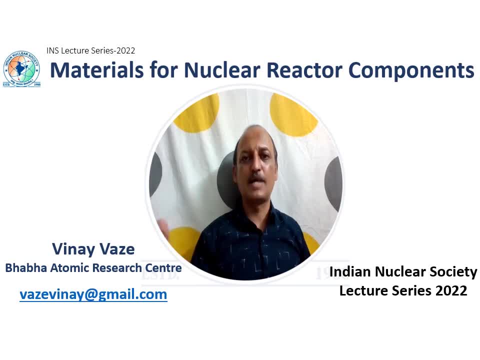 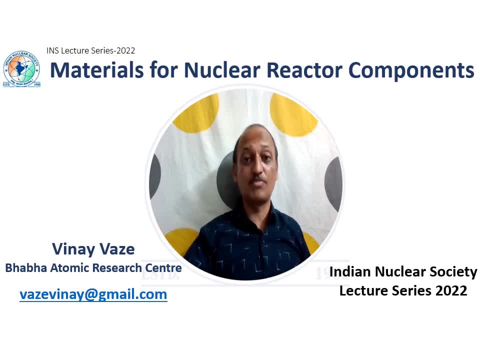 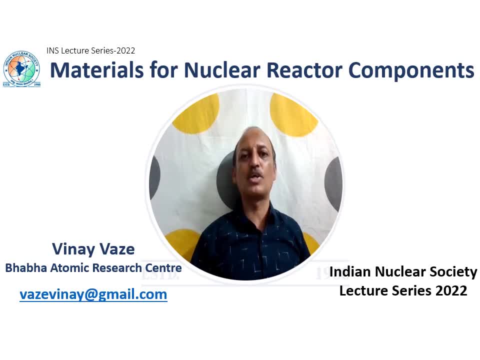 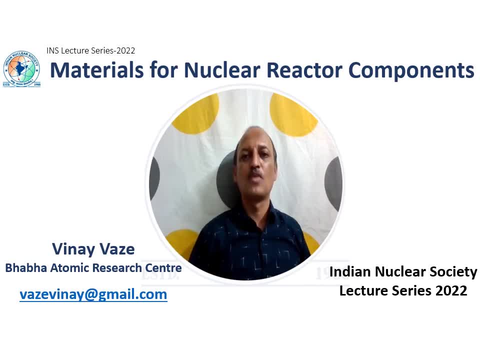 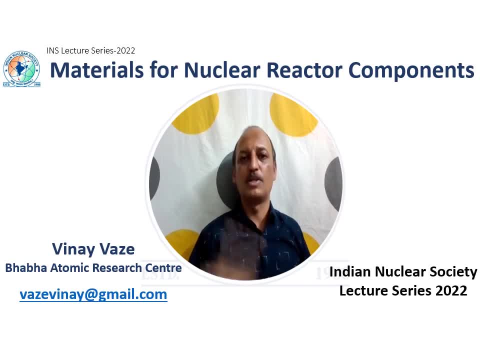 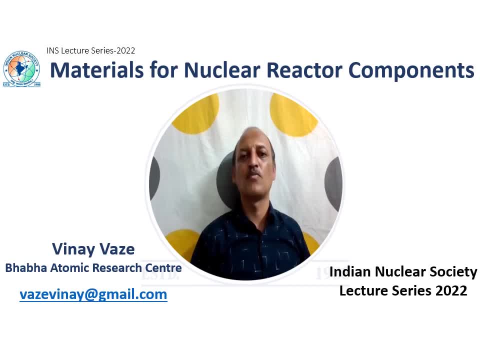 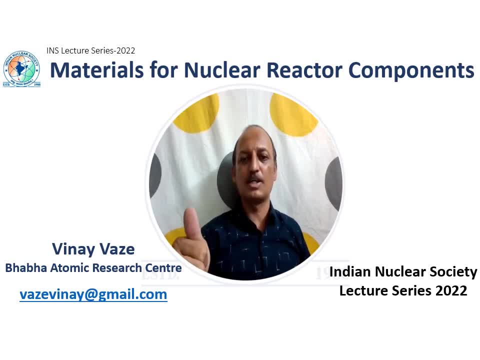 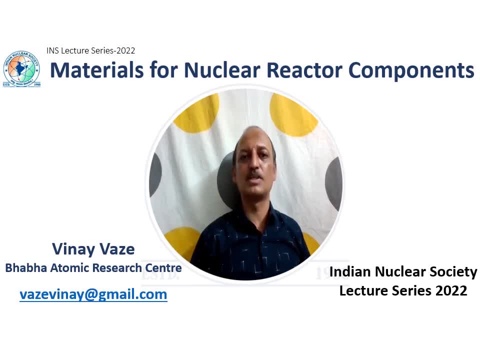 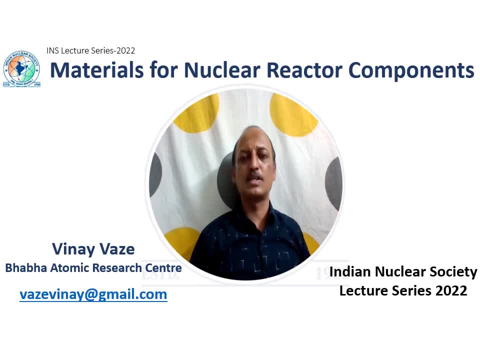 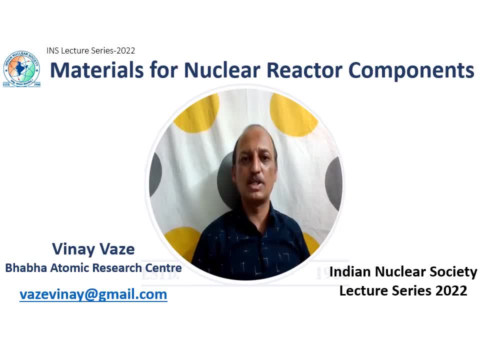 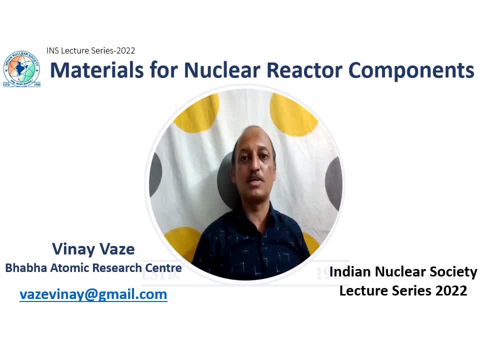 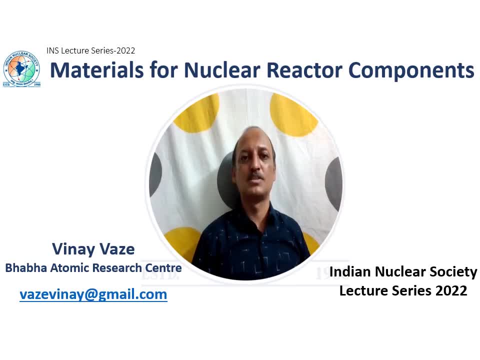 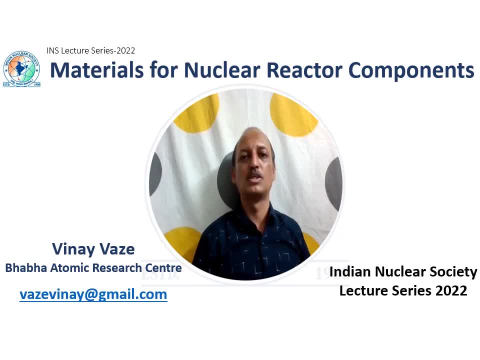 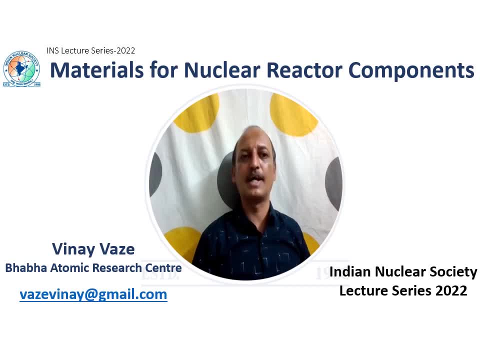 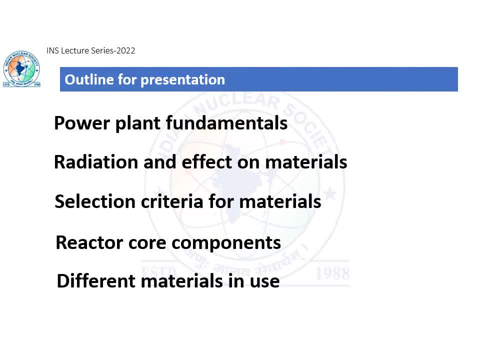 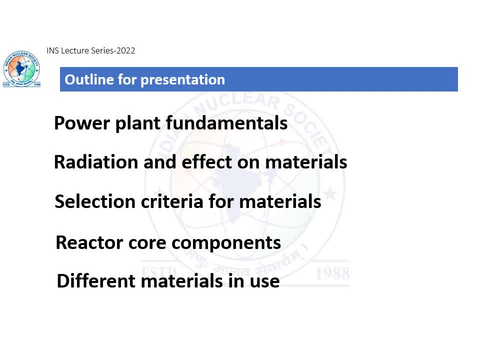 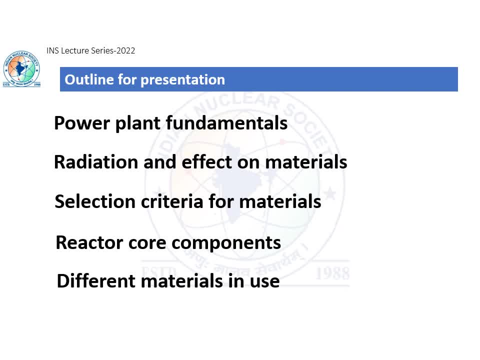 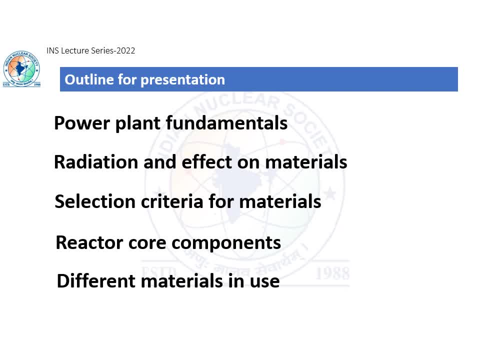 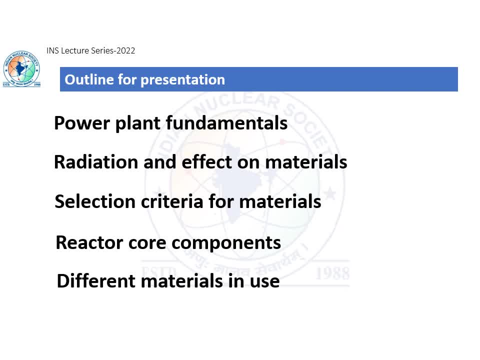 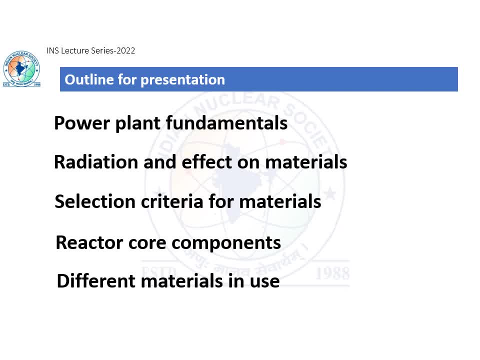 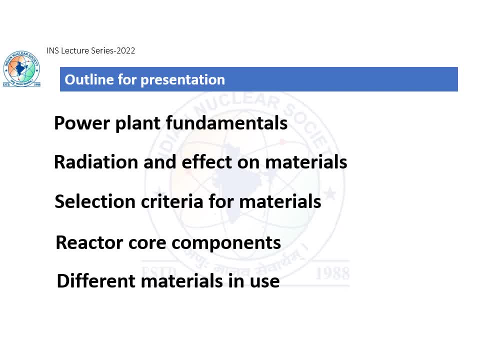 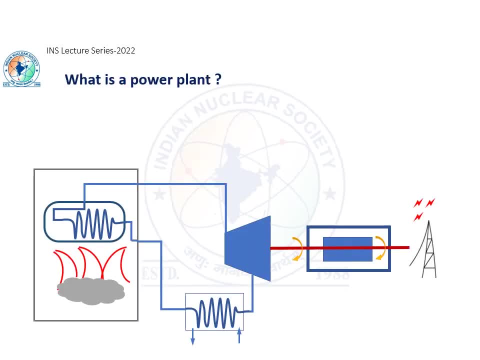 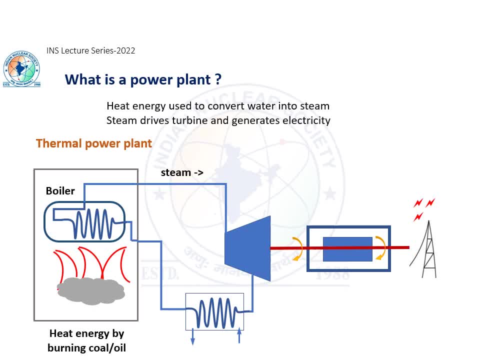 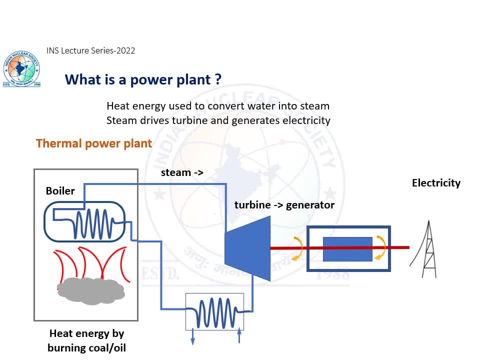 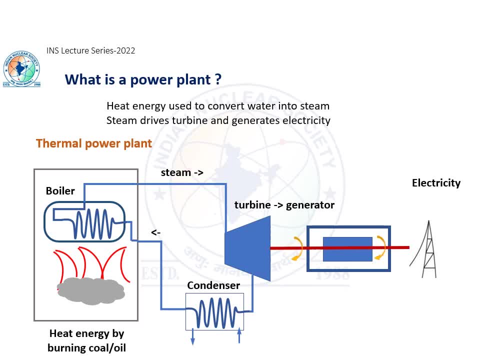 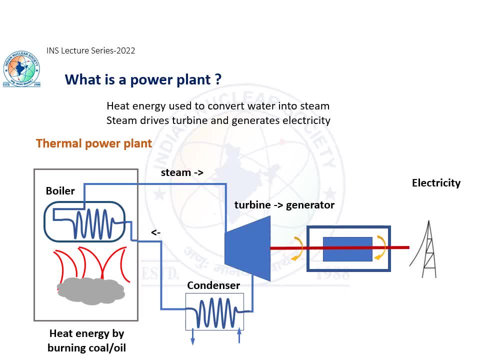 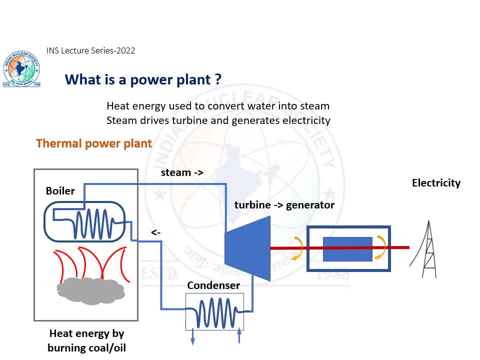 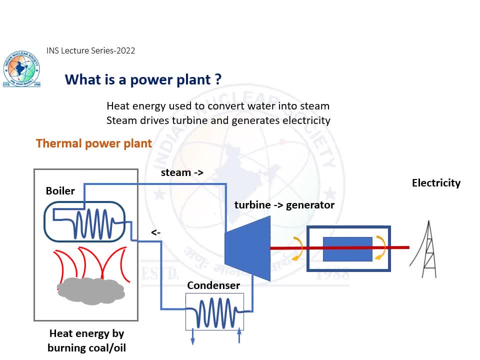 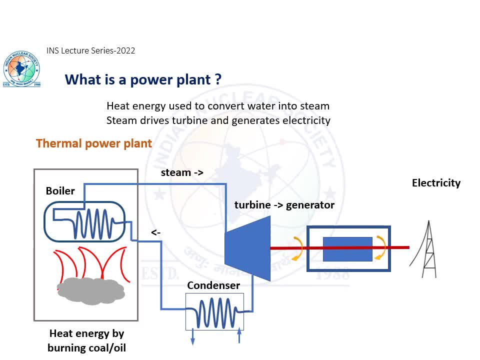 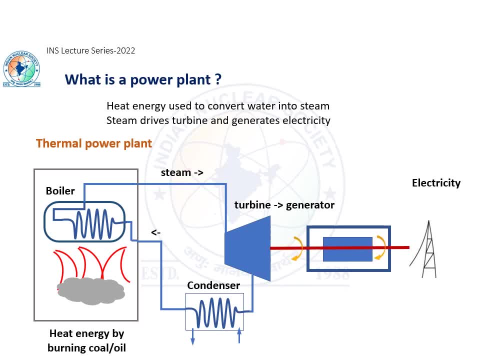 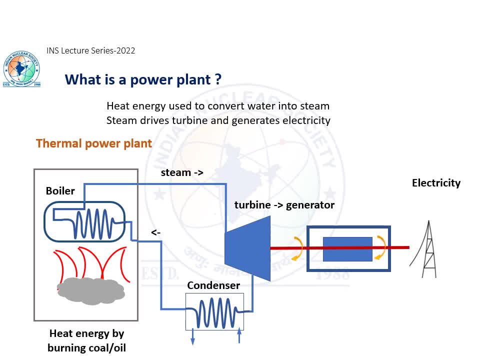 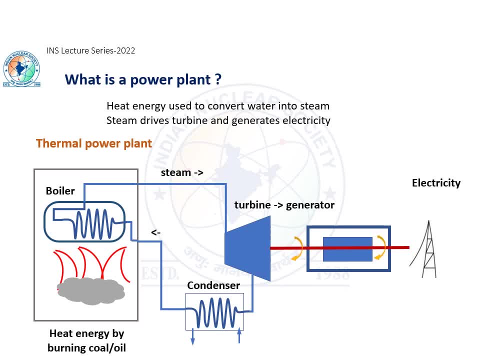 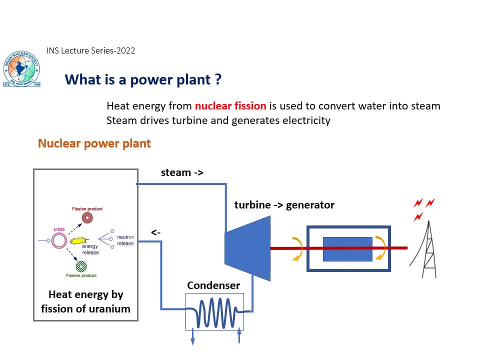 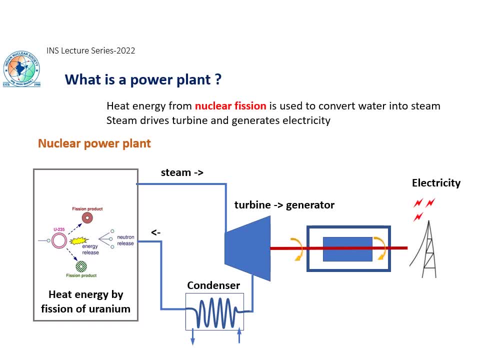 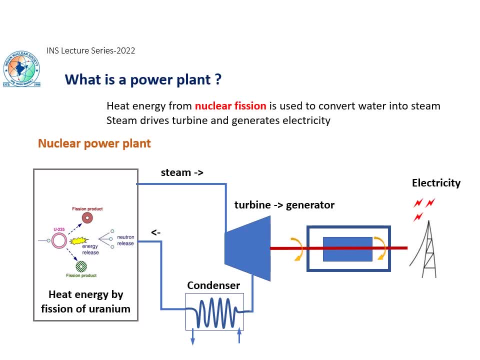 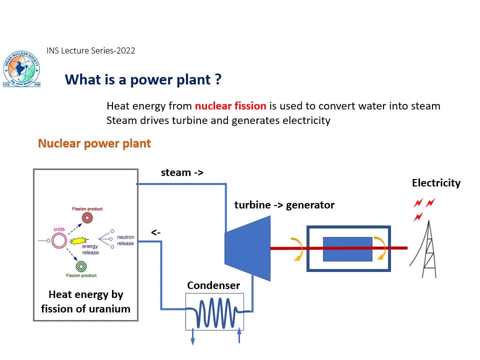 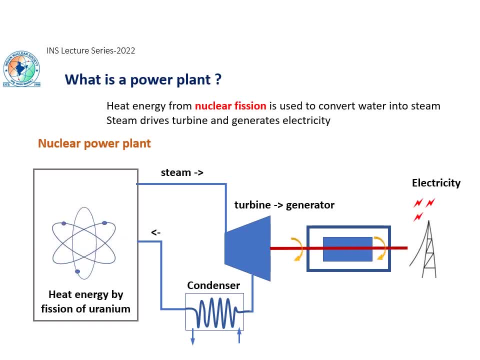 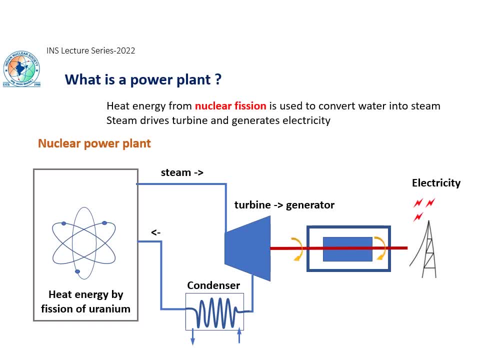 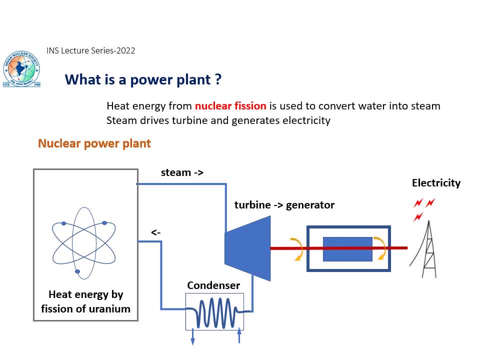 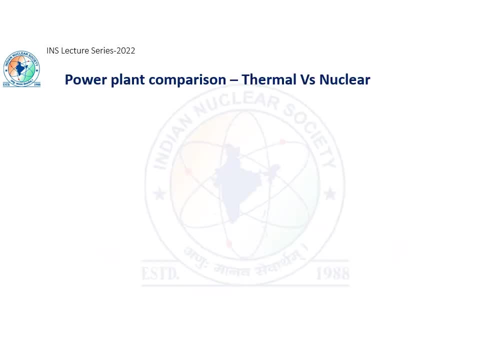 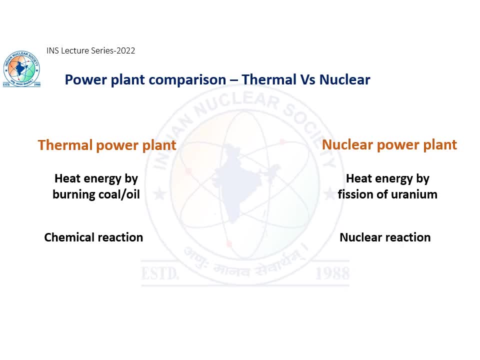 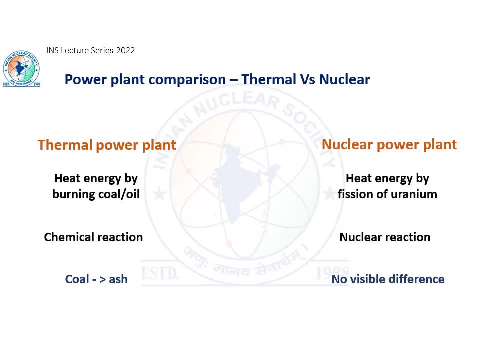 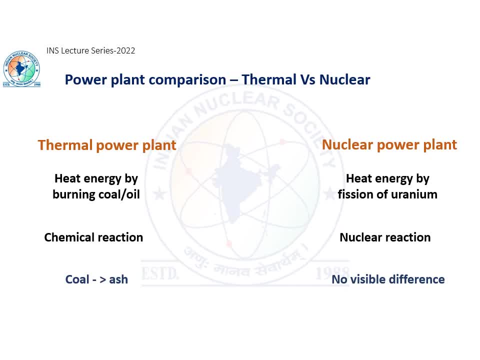 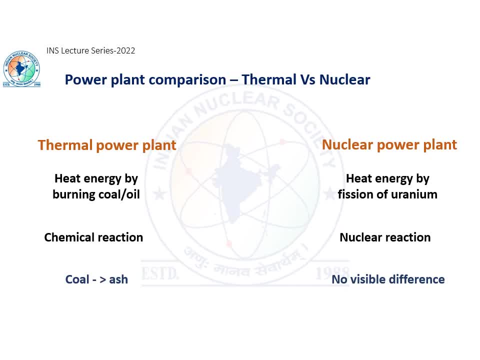 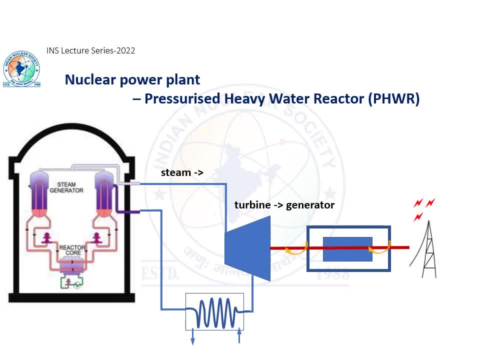 After moving through the fundamentals of Power Plant, Let us go inside the nuclear power plant. We will discuss about Indian PHWR, that is, Pressurized Heavy Water Reactor reactor. Here we see reactor building which is a civil structure housing all the necessary 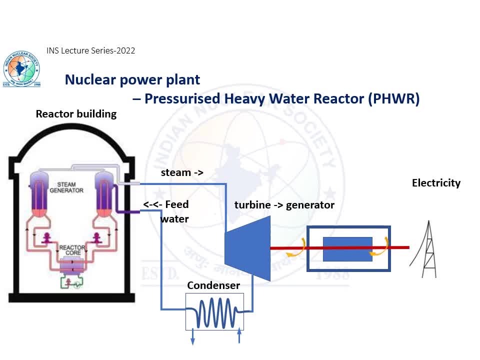 equipment, process piping and reactor core. Typically it is about 40 m in height. that is equivalent to approximately more than 10 storied of a building Reactor. core is the most critical structure and there are other associated components and systems for safe operation, like steam generator, coolant pumps, shutdown system, emergency core cooling system. 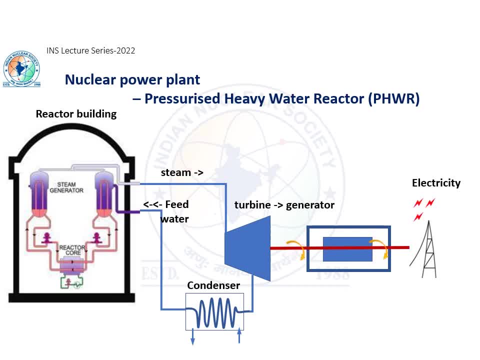 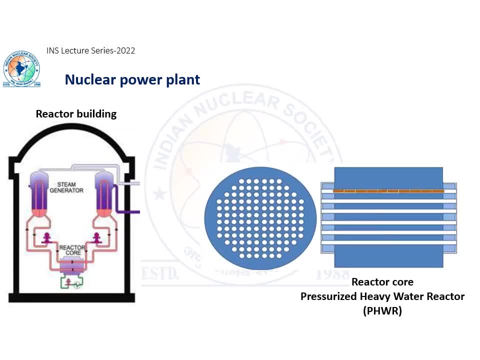 fuel handling system and fuel transport system, etc. This shows a typical reactor core configuration for Indian fresherized heavy water reactor. It is a cylindrical shaped structure with about 6 m in diameter and about 7 m long horizontal orientation. We have 18 such reactors of different power. 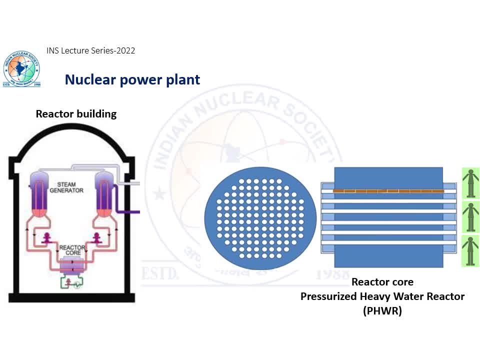 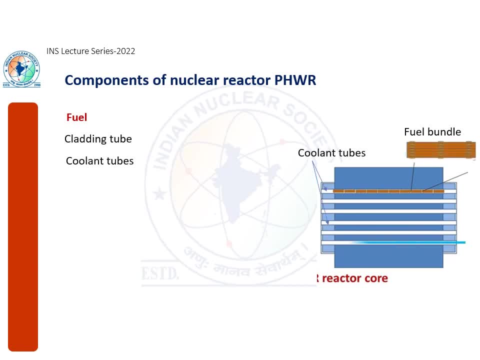 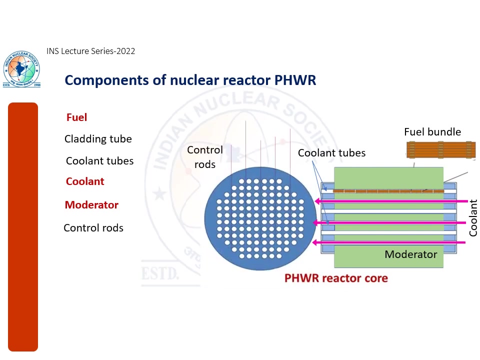 capacities located in the various parts of the country. A typical nuclear reactor core contains fuel coolant moderator as the main constituents. These materials mainly decide the type of reactor. Indian PHWRs have horizontal coolant tubes through which the coolant flows in the reactor. There is a moderator surrounding these coolant tubes. Control rods are neutron. 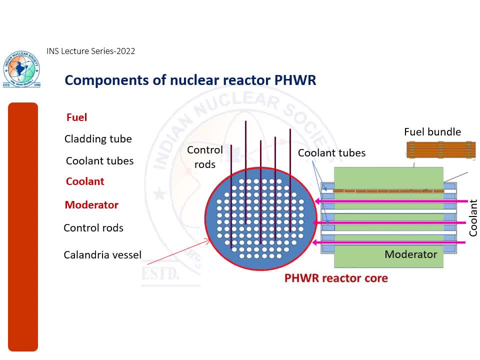 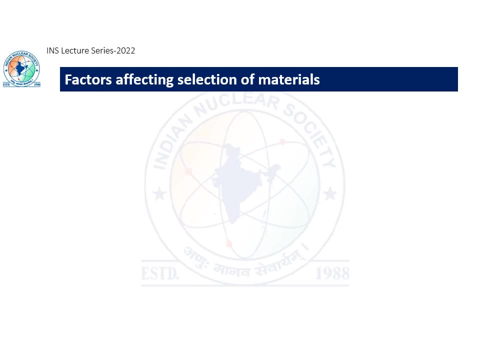 absorbing materials that control the chain reaction and thereby the fission power in the reactor. All these components are enclosed in a structure known as calendria vessel. The selection of materials is affected by many parameters or the factors. First factor is the operating conditions in the reactor core, like pressure, temperature. 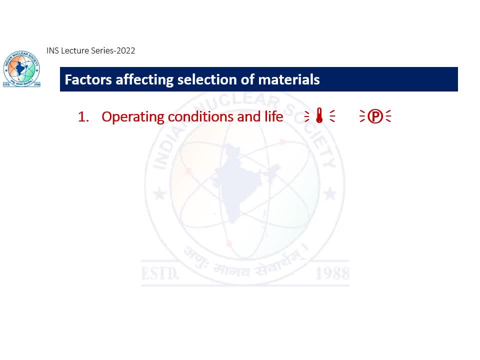 radiation, etc. that affect performance of a component. Typically, a nuclear power plant is designed for 40 years and some advanced designs even for 60 years. The next factor is degradation mechanism that limits the use of component or the materials in the core. 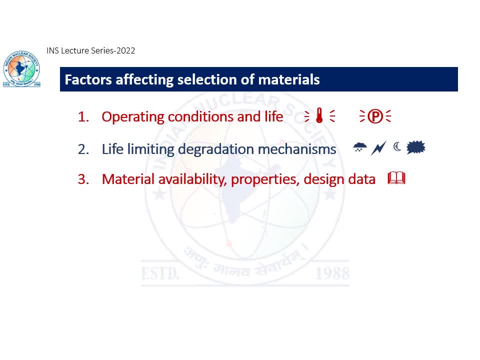 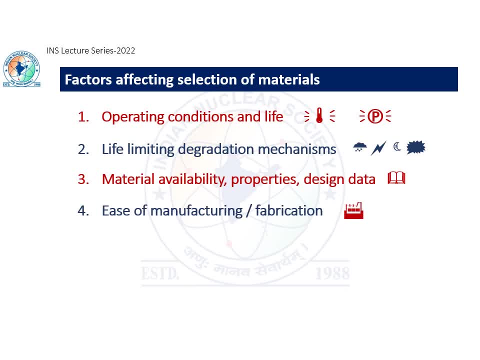 the material property data for design calculations, safety studies and regulatory documents. According to the ICJA水, Corey fowler said that two convinced engineers that nuclear grade materials are not available and not capable of operating. In addition to availability, the material shall be easy to fabricate or manufacture. 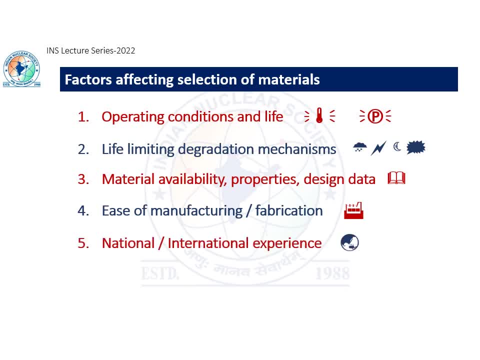 into the components, which have dimensions ranging from very small, like 1 cm or so on, to very large- 6-7 m. Therolling time of a material shall vary from 5 to 15 days on a regular basis. Existing experience of the same material components in national or international domains is also. 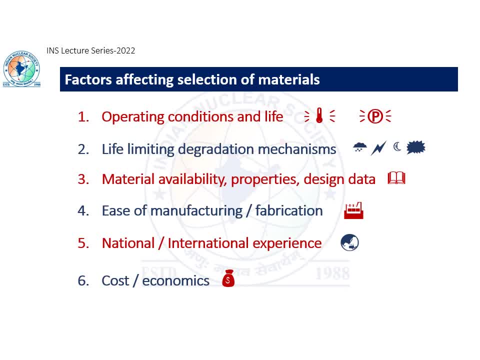 helpful for improving the understanding and its performance behavior in reactor core. Ultimately, every component material fabrication process has to be at reasonable cost, ie economics is also important. Thus the choice of materials for core components and non-core components in a reactor depends. 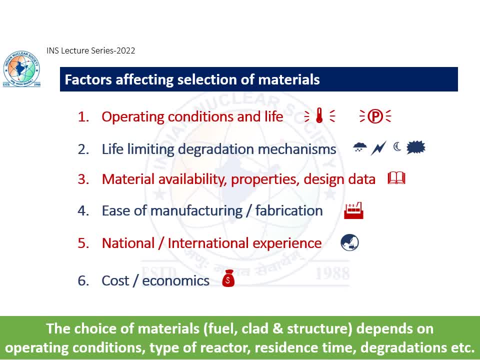 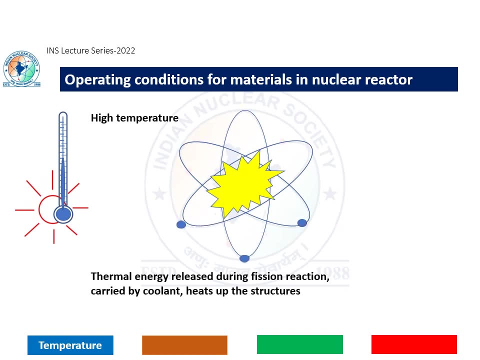 on operating conditions: type of reactor, residence, time of component in a reactor, material degradation mechanisms. Let us focus on the peculiar operating conditions which have impact on material selection. First, is the temperature: Thermal energy released during fission. reaction is carried away by a reactor coolant medium. 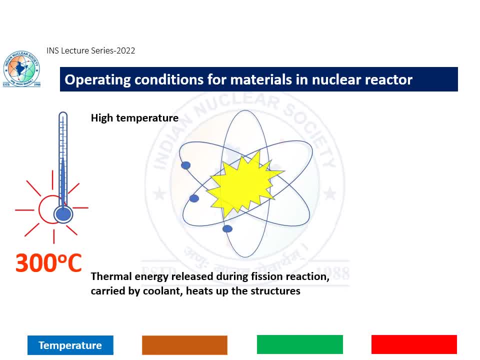 The reactor coolant in PHWR is heavy water and typically has a temperature of 300°C. This thermal energy heats up the structure and generates thermal loading. It also produces stresses on different reactor components. All the core components and the structures in PHWR are generated by thermal energy. The thermal energy is released during fission reaction and is carried away by a reactor coolant medium. The reactor coolant in PHWR is heavy water and typically has a temperature of 300°C. These Svenet 것처럼 sculptures have applied to the reactor with the help of cold humidity. 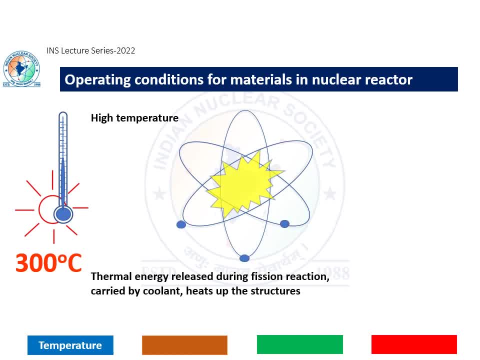 knocking out the thermal��tox sine قا. These are essentially heat and base elements of theseemas fission qu–tw, but the physically flammable temperatures have to necessarily perform well under these high temperature conditions throughout the life of a reactor, For example in: 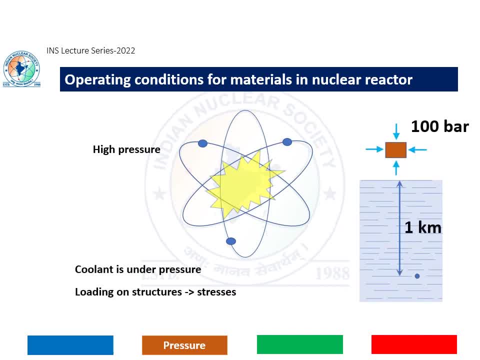 coolant pressure. Le by Med stands for external, towards its material. Then we have coolant pressure. Typical coolant pressure in the reactor system in Indian PHWR is about 100 bar. This is pressure available under water on one can experience at about 100 meters depth under. 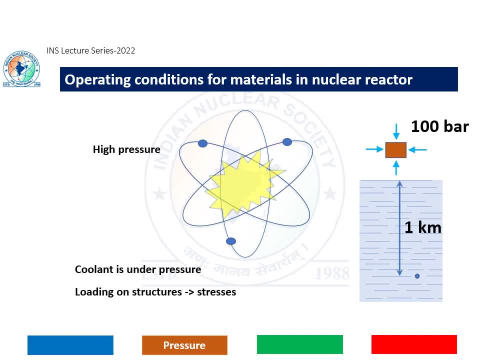 water. The forces formed by the pressure generates takeaways of much Quando we assume that there generates loading and so the stresses on different components. the structures have to sustain these stresses throughout the life for successful operation of the reactor. component corrosion is one of the undesirable chemical reaction of 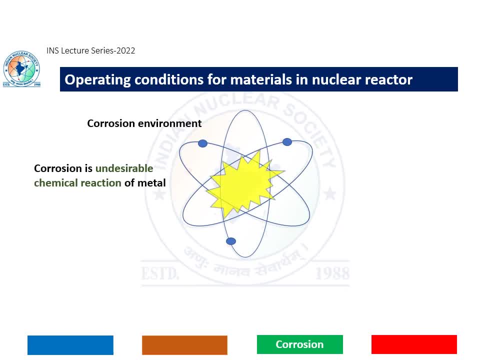 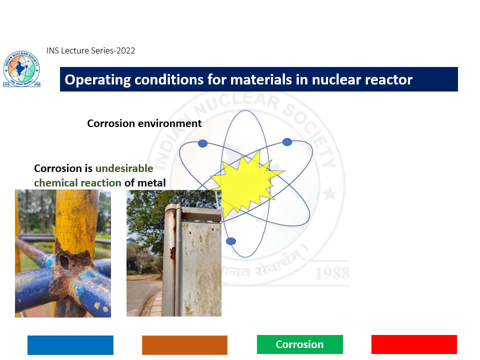 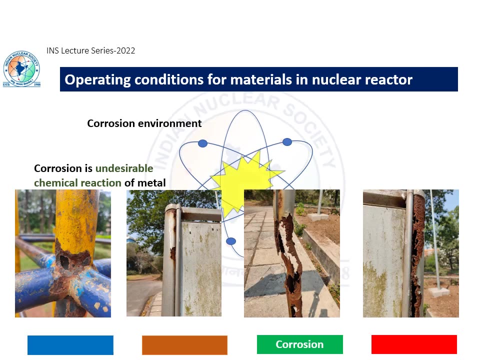 metals. all of us have seen the rusting in the bicycle spokes or wheel rim during monsoon season. that is nothing but corrosion. corrosion is basically effect of surrounding environment on material by its chemical reaction. these are some of the photographs of corrosion of metal under Sun, air or rain in open. 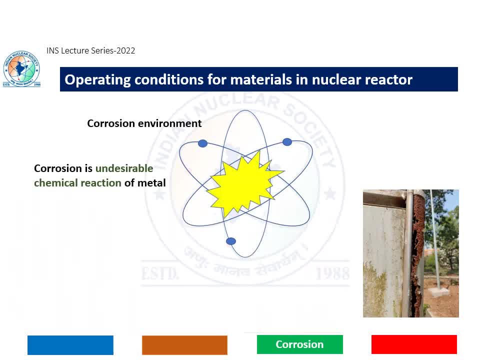 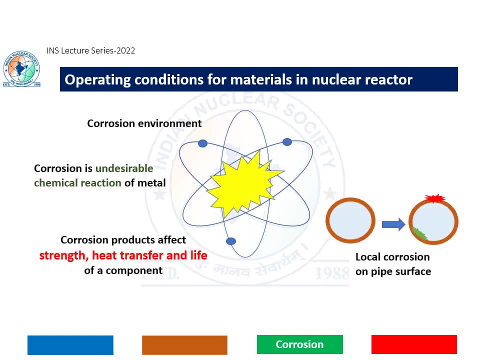 atmosphere. the corrosion products formed are most of the times undesirable because they reduce the strength of the original metal. it affects the structure of the metal and it affects the structure of the metal. it affects the heat transfer. this has impact on performance as well as life of the component. corrosion can be localized or uniform over surface. it can be seen. 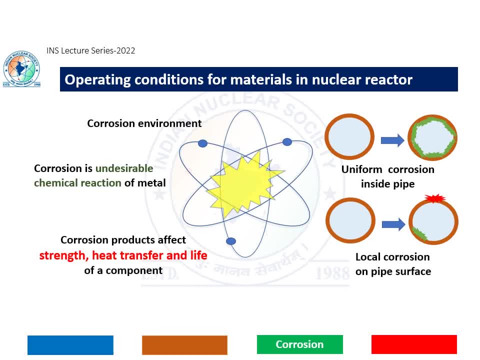 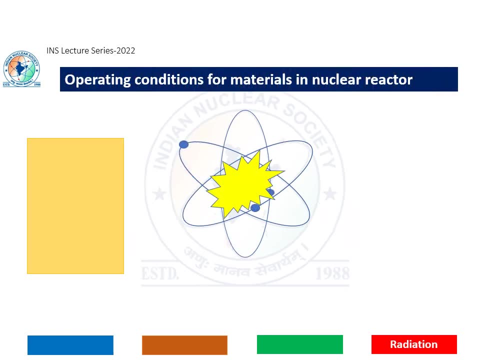 in the picture. it could be inside the piping or outside the piping, so proper measures have to be provided for avoiding or at least reducing the corrosion in the reactor core components. as we have seen, typically nuclear reactor operating conditions include high pressure, high temperature or corrosion environment, and these are 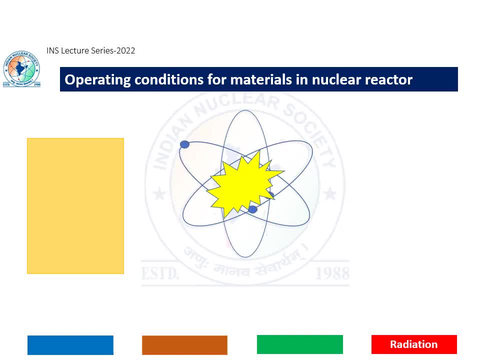 experienced in any other industrial activities also. however, it is the radiation environment that separates the nuclear industry from other industries. radiation cannot be seen, cannot be felt or it cannot be experienced like pressure, temperature or corrosion. there are different types of radiations, like alpha, beta, gamma, alpha particles are 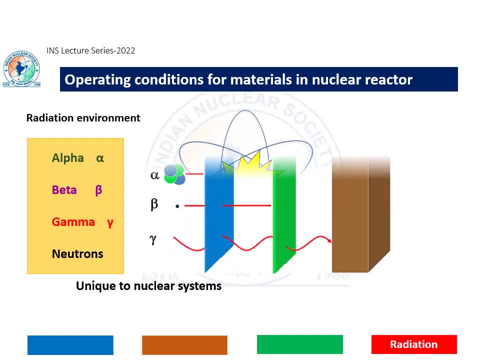 positively charged and can be stopped by a simple paper. as we can see in the image, beta radiation can be stopped by plastic or cloth. gamma rays require high density materials like concrete or steel or lead as shielding material. all the materials have neutrons as subatomic particles, and these neutrons 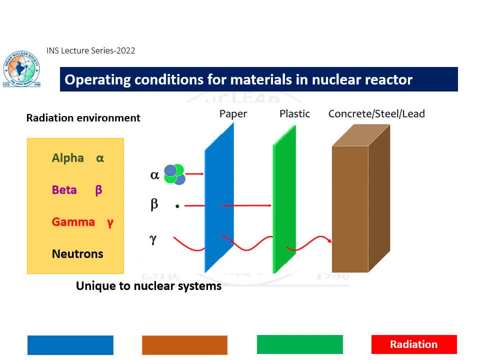 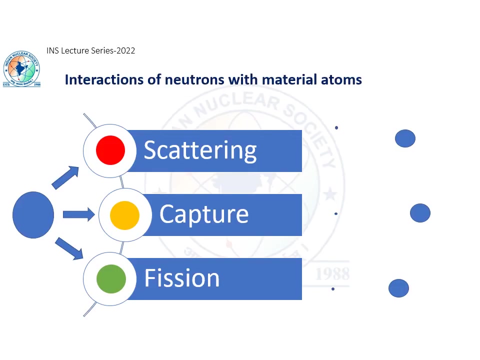 are electrically neutral. these different types of radiations with different energy levels are present inside a nuclear reactor system. the material has to perform well under radiation environment as per the design for the intended period of operation. a neutron is a subatomic particle. it does not carry any charge and it can interact in three 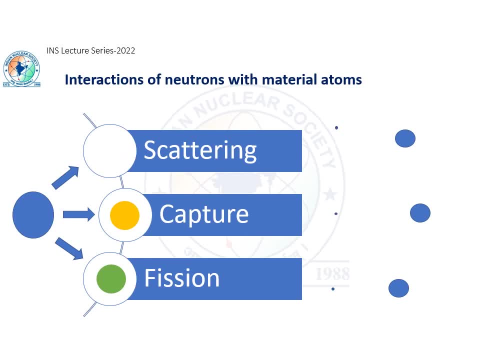 different ways with the material atom. in case of scattering, the neutron interacts with the atom and there is only exchange of energy. this is like a billiard ball collision: the atom may go to excited state or in a different energy state. in case of capture, the energy is absorbed in the atom and this forms a new isotope. 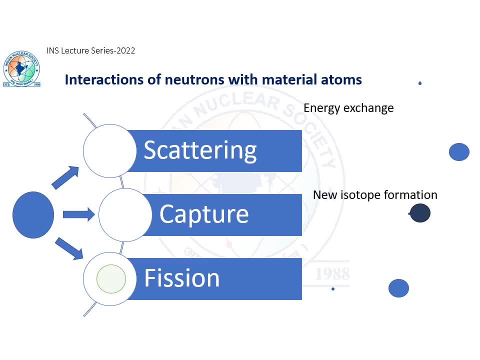 of that material. in case of fission, the neutron strikes on the atom and the splits into the atom into two lighter elements. this reaction releases three neutrons and heat energy. the neutron interacts with the material depending on the energy level and the probability of particular type of interaction for the 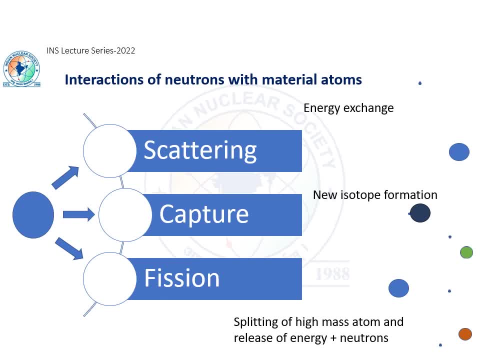 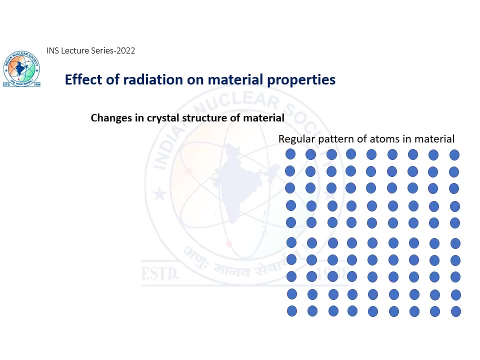 material under consideration. for example, uranium atom have high probability of fission reaction when it sees a slow energy. neutron, boron or cadmium atoms have high probability of capture reaction or absorbing of the neutron. let us now see effect of radiation on material properties. typically, a crystalline solids show a regular pattern of atoms arranged in the material. 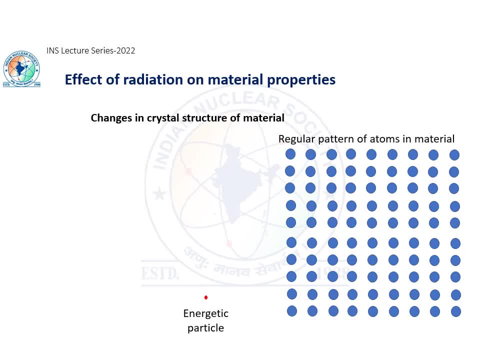 when an energetic particle comes and interacts with the atoms, and if it has sufficient energy, it can dislodge the atoms from its regular position. this creates a vacancy, that is, absence of an atom at its regular position. if the particle has sufficient energy for the contact with the material, it can continue to do so and create some more. 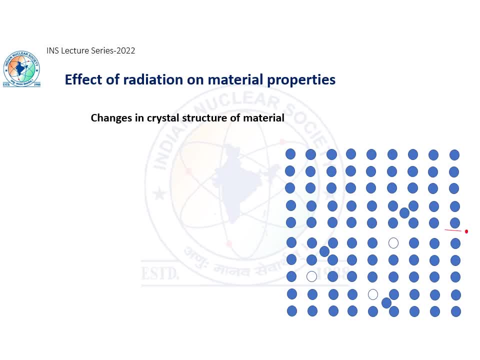 vacancies in the crystal structure. it can continue to do so till it comes in equilibrium with the material structure. so there are number of vacancies created by radiations. in the same way there are number of interstitial entities, and in the same way there are number of interstitial entities and in this way, a 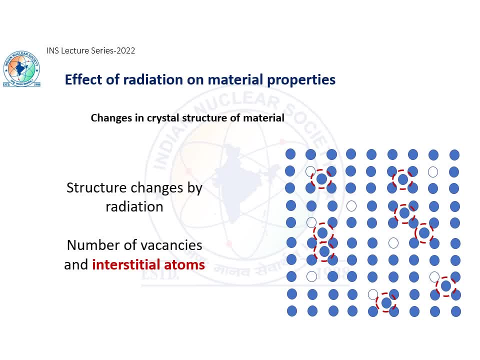 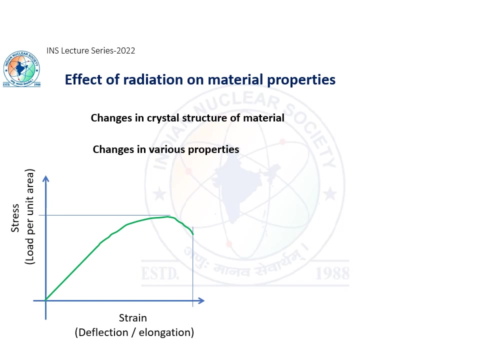 atoms are created. so these are nothing but the atoms which are displaced from their other locations and they are now occupying a place where they should not be. so vacancies and interstitial atoms: these are the structural changes that are done by radiation. now we see the changes in various properties of material. 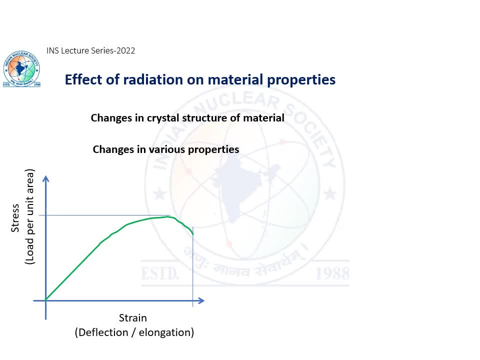 because of radiation. first, let us try to understand the fundamentals of these basic properties. this is typical stress versus strain graph for a material, as you can see on the screen. strength is the maximum load that it can sustain or resist for a given deformation. elastic modulus or the young's modulus, as we have studied in our college. it shows the 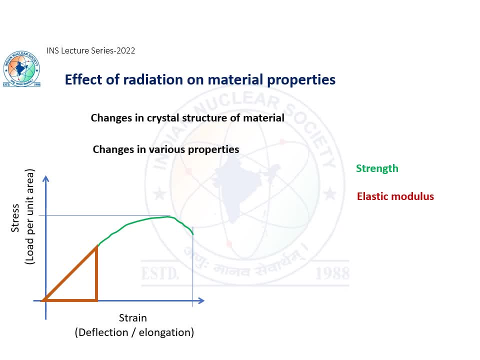 linear dependence of the load and deflection, that is, if the load is doubled, the deflection will be double. thus there is a linear relationship between the load and the deflection. then toughness is the area under stress strain curve as shown by the shaded region, higher the 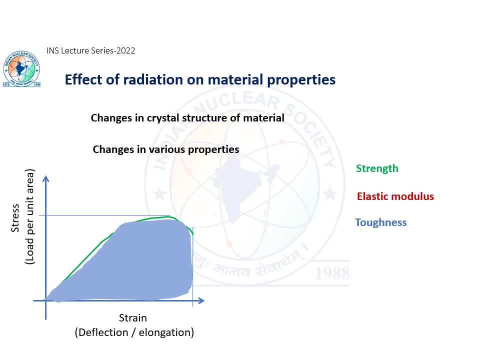 toughness, higher is the capacity of the material to withstand the sudden or shock loads or the impact loads. ductility is the ability of the material to be drawn into wire. so how these properties are affected by radiation. with radiation exposure, the material strength in the structure of the system increases. that is component can sustain higher loads. the elastic. 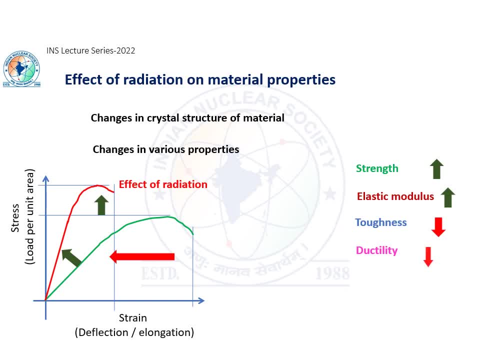 modulus increases, while the toughness and ductility reduces under iridation. this means the capacity of component or the material to take the shock load is reduced. also, its capacity to stretching like elastically, like rubber is reduced. thus, as a result of radiation, some of the properties increase, starting at the source. 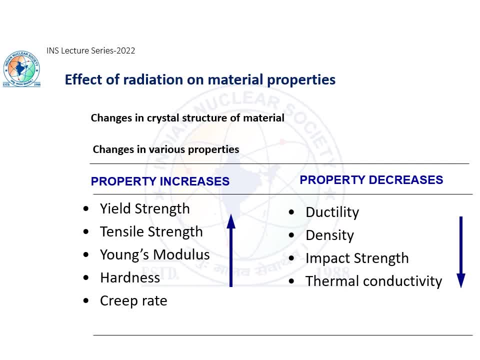 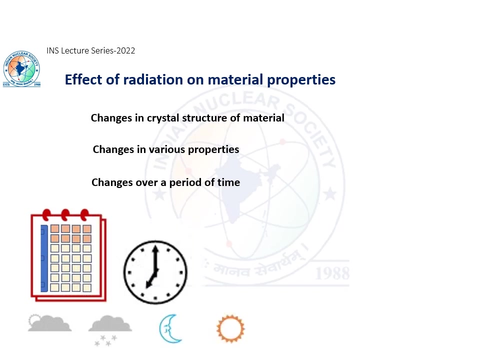 like yield strength, tensile strength, Young's modulus or elastic modulus, hardness and creep rate. Then some of the properties decrease as a effect of radiation. These include ductility, density of the material, impact strength and thermal conductivity, etc. When the radiation affects the material properties, it generally happens over a period of time. 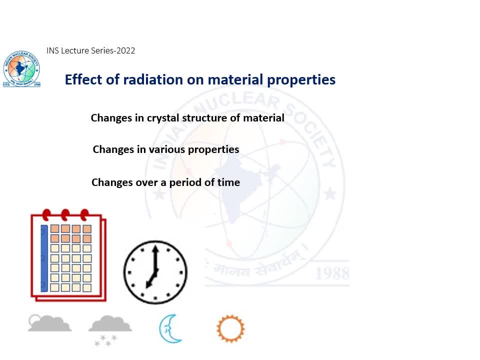 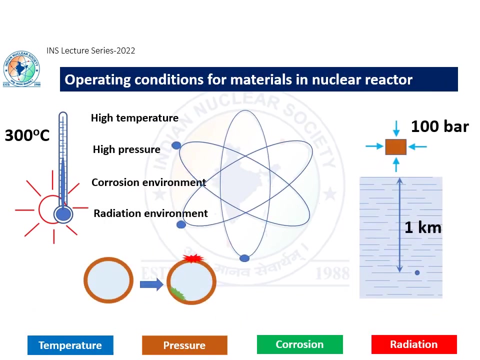 Typically, a nuclear reactor is designed for 40 years, and some advanced designs have a life of 60 years. The time frame over which these changes occur in the materials due to radiation are typically much higher than the lifespan of the reactor components. So, to summarize, we see the operating conditions for a nuclear reactor. 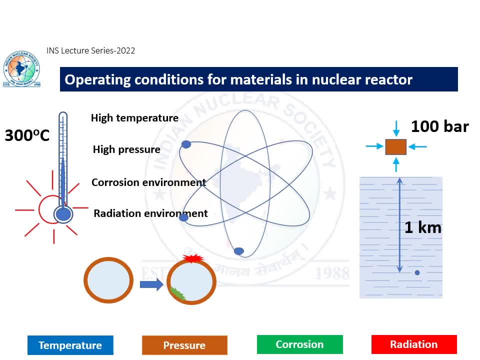 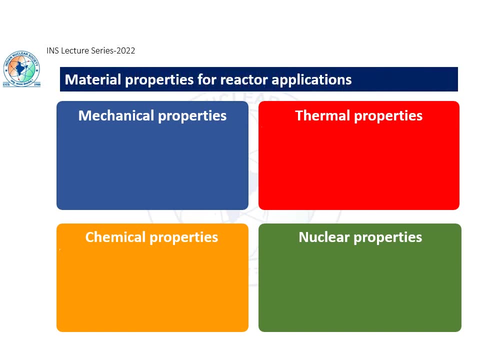 We have high pressure, high temperature, corrosion environment and radiation environment, which is seen by the materials or the components in the reactor core. Now, with this background of operating conditions for the reactor core, let us see what are the desirable technical properties for the materials. Mechanical properties tell about strength. 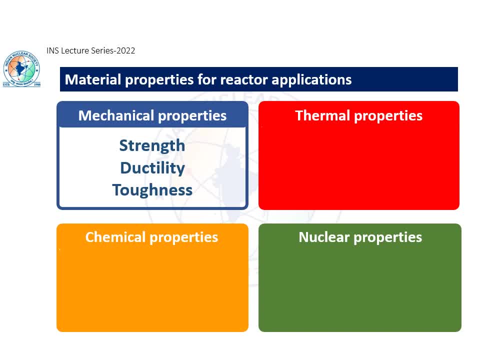 ductility, toughness or hardness. High strength of the material helps against the forces of the loads during operation. High ductility ensures the material can retain the stretching properties, like rubber, to accommodate operating loads. High toughness helps in sustaining the impact loads or the shock loads. 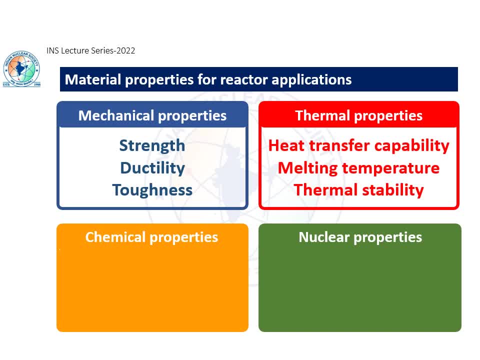 Thermal properties govern the behavior of component at elevated temperatures. High heat transfer rates, high thermal conductivity, higher melting temperatures and good thermal stability are important requirements for material to perform at elevated temperatures. When it comes to chemical properties, the compatibility with the other structural materials, 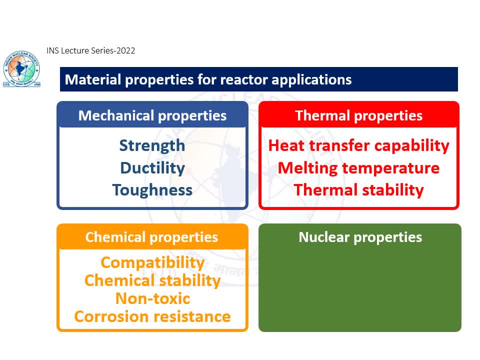 material stability under operating conditions, non-toxicity and good corrosion resistance become very important for better performance of the component. All these, either independently or together, may be required in other industrial applications, But nuclear reactors or their components, in addition to all these properties, have unique 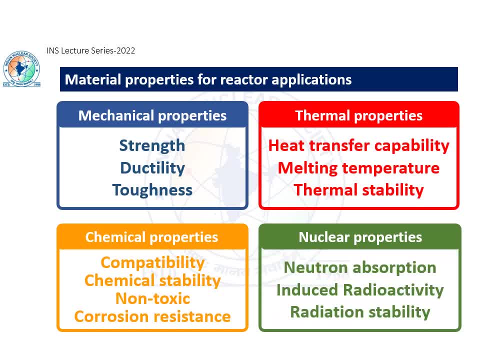 requirement of material nuclear properties. These include the low neutron absorption capability, low induced radioactivity and good stability under the radiation environment it sees in the reactor core, The nuclear properties mainly decide the use of a particular material for a specific function, for a component. 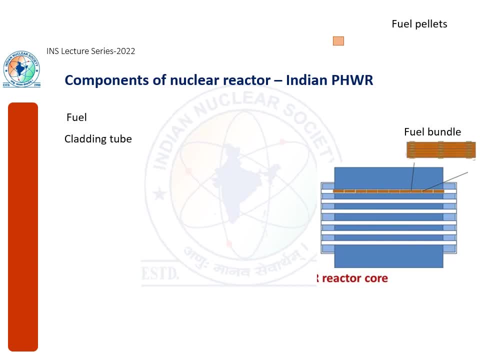 After seeing the operating conditions for reactor core and desirable material properties for components, let us revisit the different components. Let us see the operating conditions for reactor core and desirable material properties for components. There is a component name of the reactor core or the nuclear property. 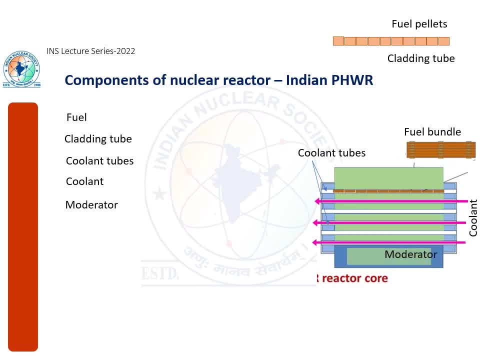 Code Eor- aproximately. it is the components that are most frequently used to perform an industrial operation. This component of the reactor core is known as the main component of the reactor. It is the main component of the reactor. When the reactor core is initiated, it is the main part of the reactor. 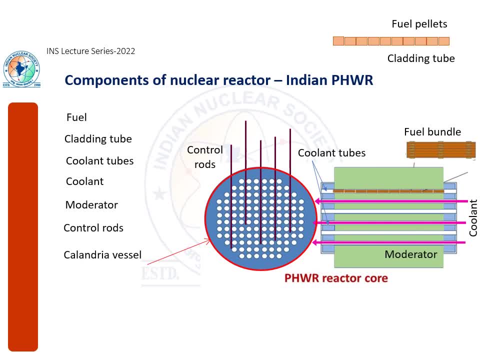 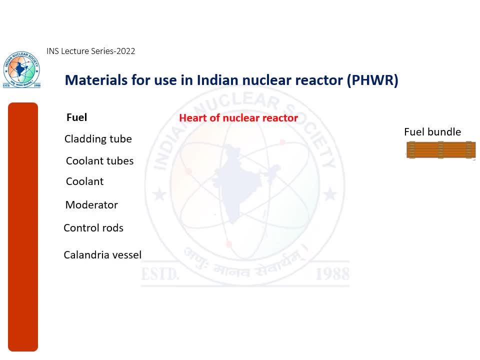 It is the basic component of the reactor. go into the details of each of these components. fuel is heart of nuclear reactor. nuclear fission reaction is happening in fuel material and energy is released as heat. uranium is commonly used fuel material in its oxide form in almost all the thermal power reactors worldwide. for 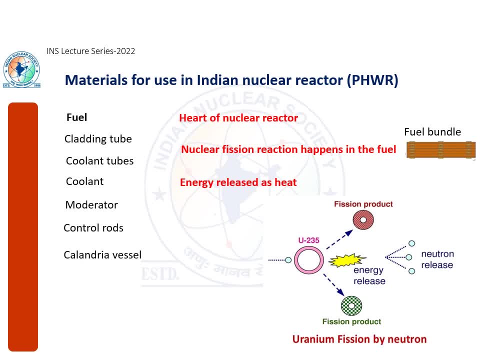 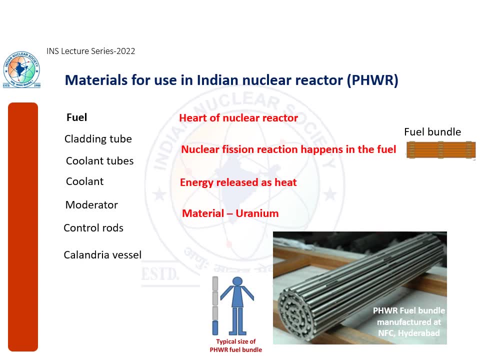 last more than five decades. typical fuel bundle for PHWR is about half a meter length and has a diameter of around ten centimeter. as you can see in the picture, number of such fuel bundles are placed inside each of the coolant tube for the reactor core in PHWR. 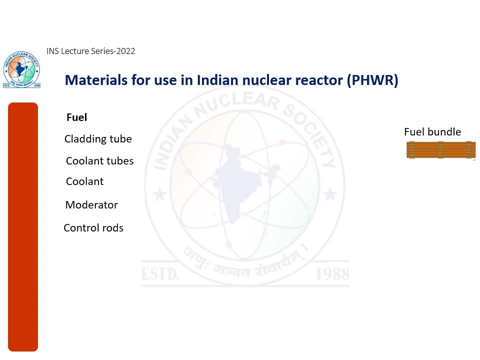 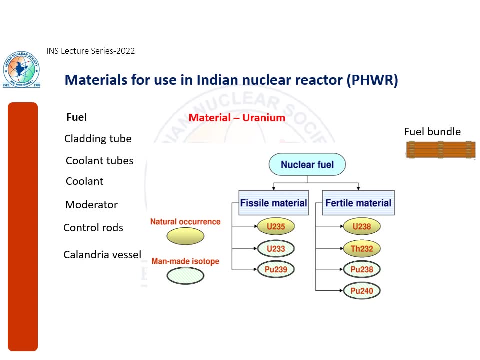 the fuel material is uranium, uranium 235, plutonium 239 or uranium 235 and plutonium 238, which 233, are fissile materials that are suitable for chain reaction in nuclear reactor. only uranium 235 has natural occurrence. that too very low. the other two isotopes are produced after neutron irradiation of uranium or thorium in. 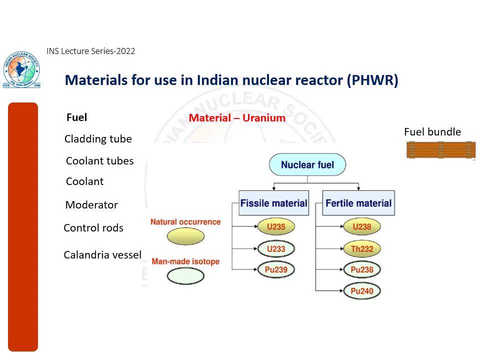 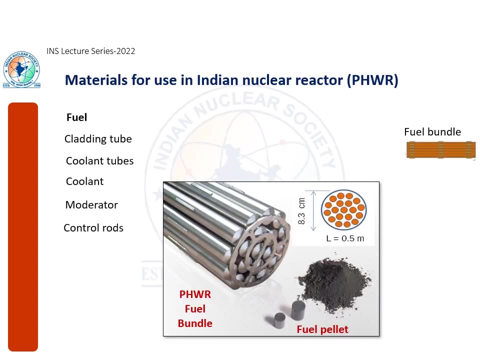 reactor core. uranium is commonly used fuel material in its oxide form in almost all the thermal power reactors in the world for last more than five decades. here we can see uranium dioxide fuel bundle. the raw material is uranium dioxide powder and it is processed by thermo mechanical techniques to make high-density fuel pellets. these pellets 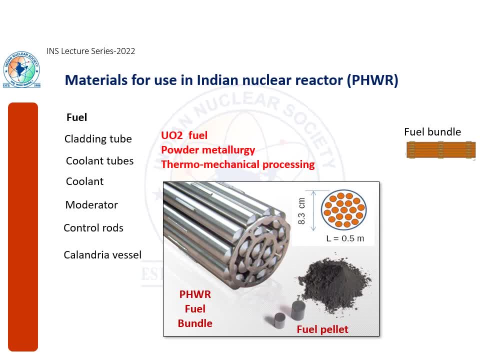 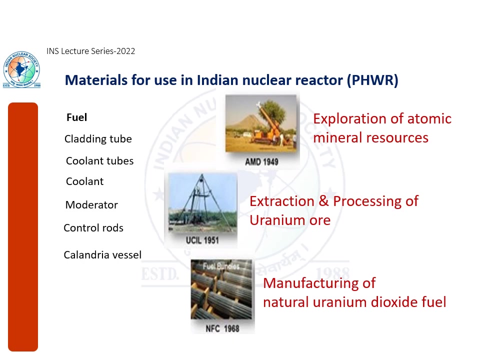 are filled in cladding tube, sealed at both ends, and such number of fuel pins are assembled together with structure components, like in plate, to form a fuel bundle. number of such fuel bundles are placed in each of the coolant tubes of the reactor core. the atomic mineral direct rate carries out activities on exploration of atomic mineral resources. 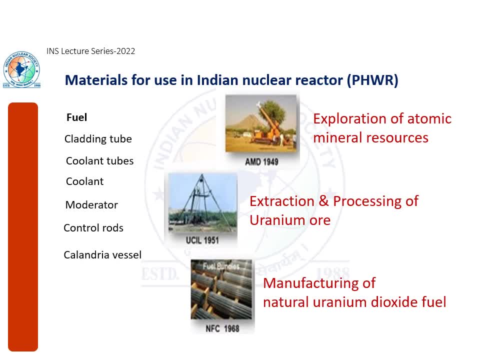 in India. that is, basically they try to identify the locations for nuclear materials like uranium, once these are studied for scientific and economic purposes. the extraction and processing of these uranium ore resources from mines is carried out by Uranium Corporation of India, limited for UCI l all. 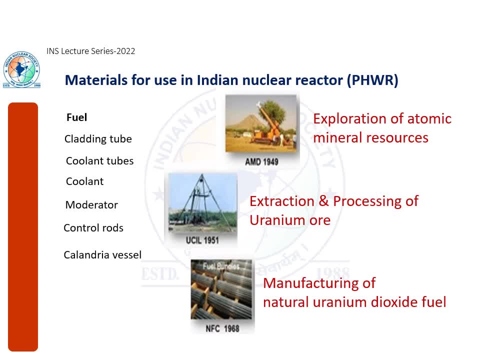 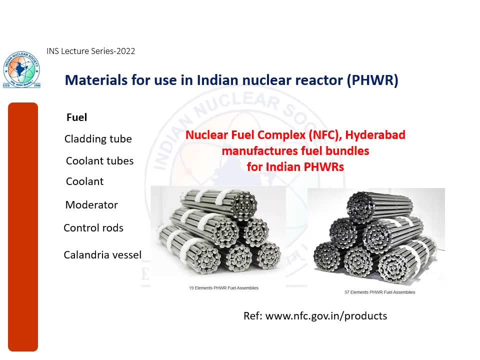 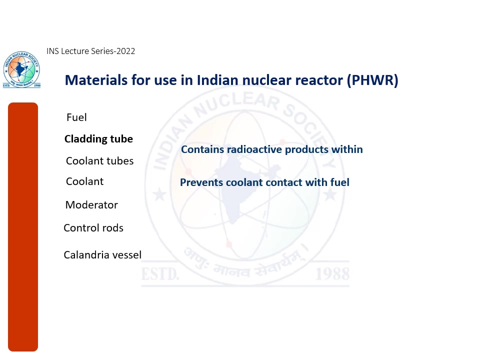 these materials are transferred to nuclear fuel complex at Hyderabad for processing and manufacturing of the fuel bundles and district quality control. the nuclear fuel complex NFC located at Hyderabad is manufacturing fuel bundles for India since 1971.. The fuel cladding is most important safety barrier in fission nuclear reactors. 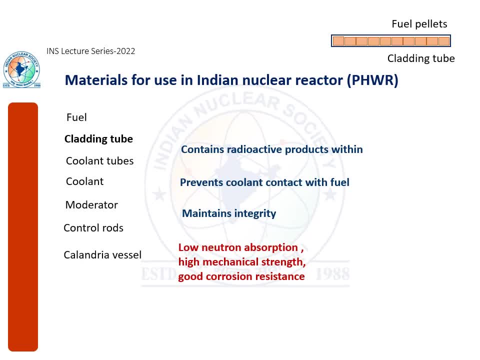 It retains most of the radioactive fission products within its volume and does not allow coolant to come in direct contact with fuel. The selection of fuel cladding material is based on many design considerations like neutron absorption, cross section mechanical strength, service temperature, good corrosion resistance. 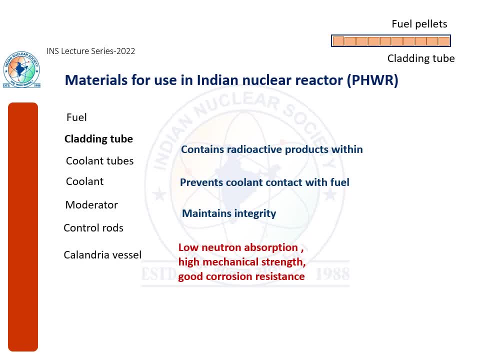 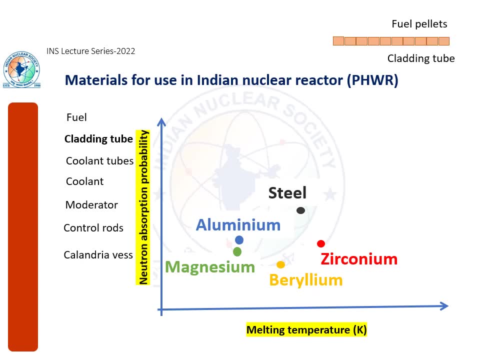 and other thermal properties. Out of all the elements in the periodic table, only four elements satisfy the requirement of materials suitable for cladding tube. These are aluminum, magnesium, beryllium and zirconium. Zirconium, being brittle and chemically toxic, can be used on a limited scale. 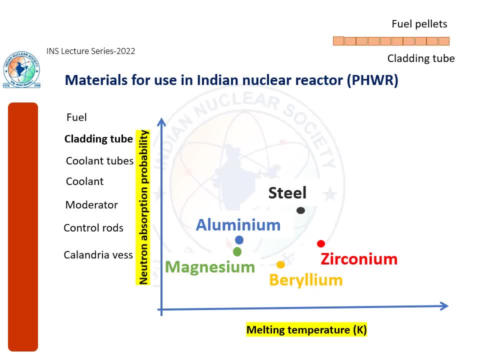 Magnesium is ruled out in water cooled reactors because of its high chemical reactivity. Aluminium has low melting point and can be used only in research reactors where temperatures are lower. Hence, for water cooled nuclear power reactors, the unique and sufficient choice is in the 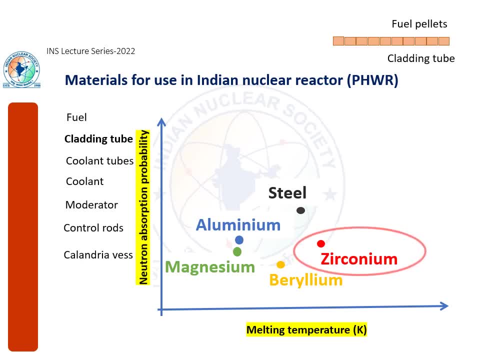 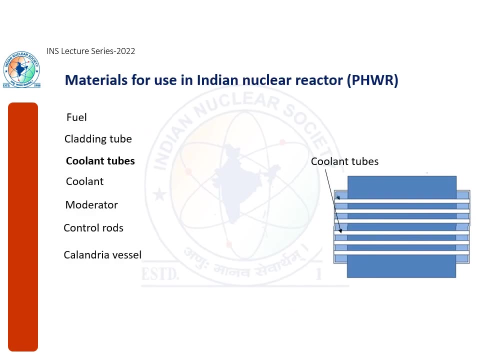 form of zirconium based alloys. Production of nuclear grade zirconium requires special technologies which has seen been mastered by only few of the countries, and, yes, India is one of them. Coolant tubes provide the passage for high pressure, high temperature coolant, which is 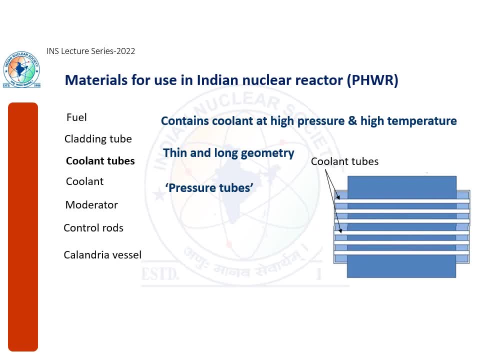 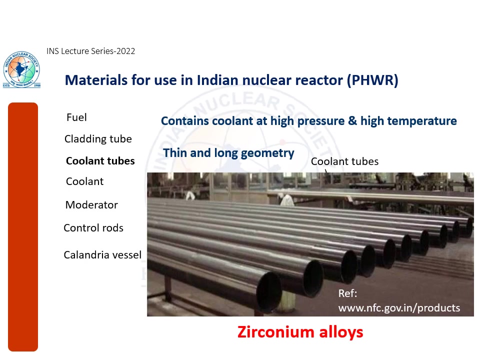 removing heat from the fuel. These are horizontal, thin and long tubes and also referred as pressure tubes in PHWRs. The material requires low neutron absorption, high mechanical strength, good corrosion resistance and creep resistance. These tubes are manufactured from zirconium-based alloys at Nuclear Fuel Complex Hyderabad. 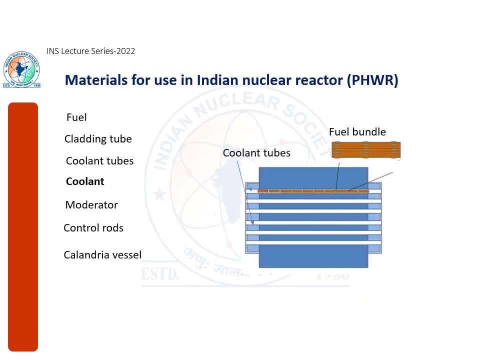 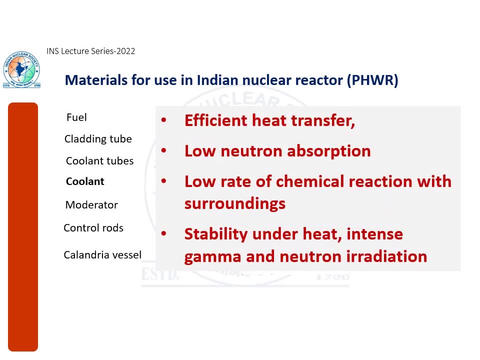 The coolant is an important component that performs the function of removing heat from heated fuel bundle during operation and transients. The material requirements include: efficient heat transfer from hot fuel. low neutron absorption in the reactor core. low rate of chemical reaction with surrounding. that is, compatibility with the structural materials. 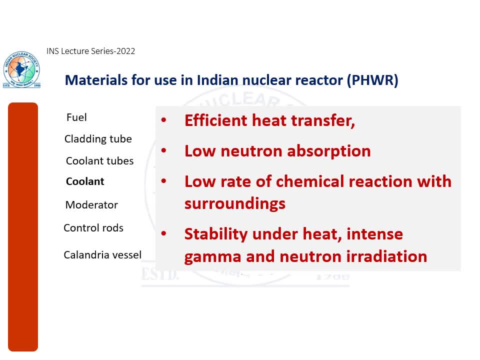 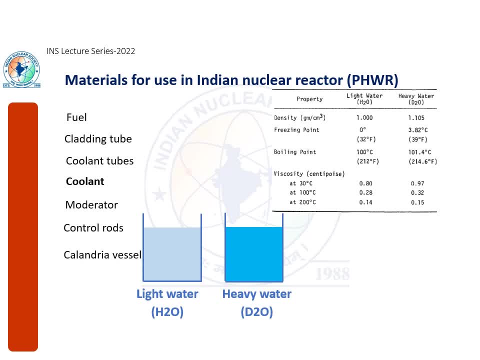 A suitable coolant is required to extract heat from the reactor. core Light water is ordinary water, which we know Heavy water is with deuterium isotope of hydrogen. It is basically D2O. It is chemically similar, slightly heavier than ordinary water, as we can see from the table of properties. 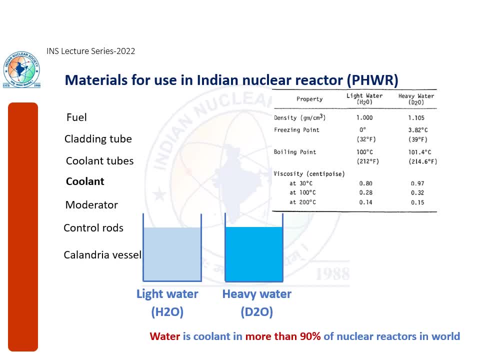 But it has very good nuclear properties. Water is used as a coolant in verse 90% of the reactors reactors. there are some advanced reactor designs that use gas like helium or carbon dioxide as coolant, or even liquid metals like sodium or lead in molten. 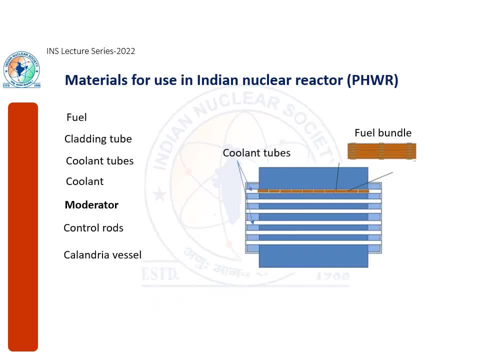 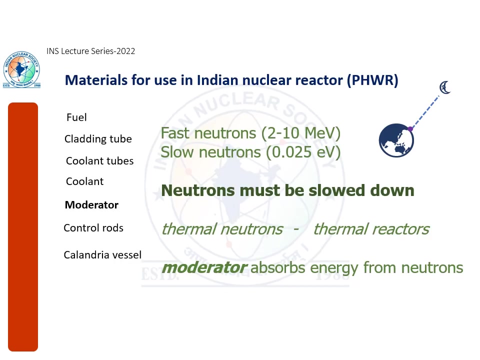 condition: Indian PHWR contains large volume of heavy water around the coolant tubes inside calendria vessel. this highlighted volume is a moderator for the reactor core. it slows down the neutrons to make them suitable to cause fission in the reactor. there are two types of neutrons based on their energy. 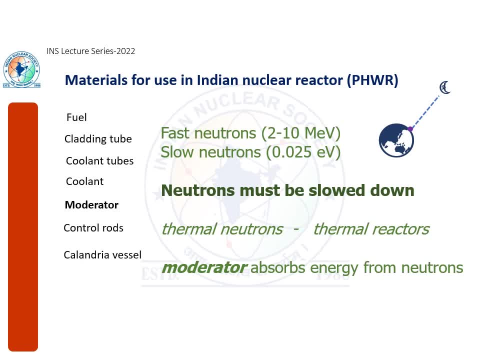 levels fast. neutrons typically have energies in million electron volts. with this energy, a neutron can travel from the earth to the moon and come back in less than one minute for one trip. the moderator material slows down these neutrons to the maximum and the neutrons can travel from the earth to the moon. 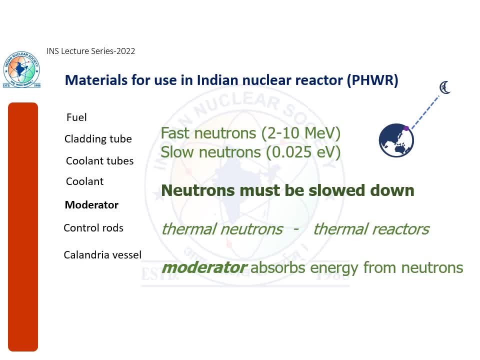 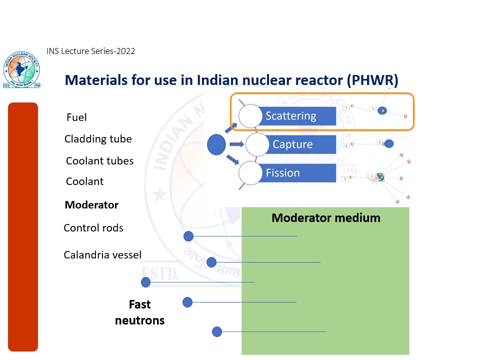 to level of electron volt range. these are called as the slow neutrons or the thermal neutrons, and the nuclear reactors based on this concept are referred as thermal reactors. thus, the moderator absorb the energy from neutrons and slows them down. the scattering reaction of neutrons is 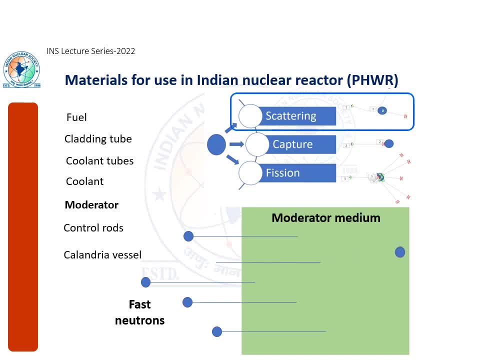 important for a material to be good. moderator in a nuclear reactor, the moderator medium, they undergo collisions and lose their energy. as we see here, neutrons of different energies are slowed down in moderating medium and these slow neutrons, or thermal neutrons, then interact with the fuel atoms to 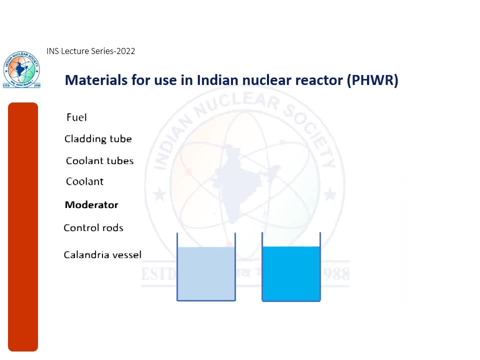 cause further fission. it is desirable to have a good scattering probability, but low neutron absorption probability for a material to be good moderator in a nuclear reactor is very important. in a nuclear reactor the material can be solid or liquid. typically light water or heavy water are used as moderators in the 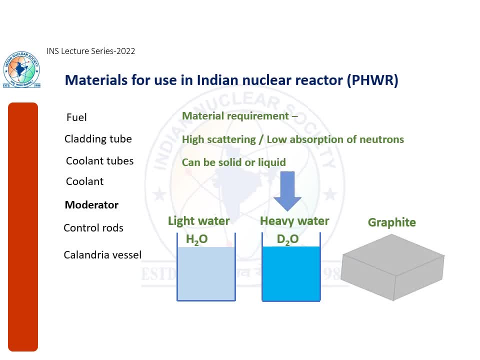 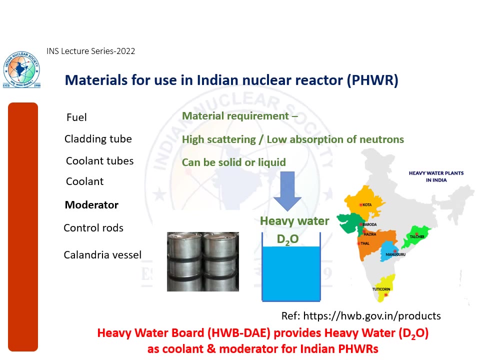 majority of the reactors worldwide. there are some designs that use graphite as moderator material. heavy water board under Department of Atomic Energy makes the heavy water not only for use in Indian pressurized heavy water reactors but also exports to some other countries. we can see the locations of different 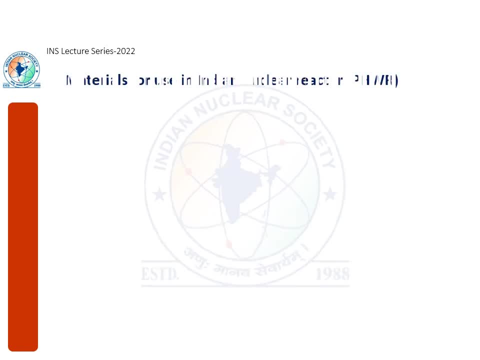 heavy water plants in India on the screen for control rods. neutron absorbing materials are used for controlling the neutron population inside the reactor core. these control rods are distributed in the reactor core volume. as we can see. these are vertically inserted from top in the typical PAWR reactor core any nuclear fission reaction produces. 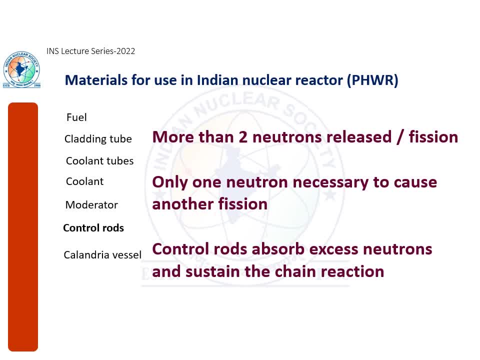 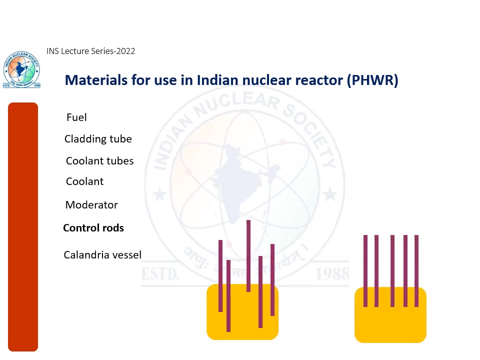 more neutrons than it consumes. more than two neutrons are released per fission reaction. only one neutron is necessary to cause fission in another atom and this continues the chain reaction. the control rod materials strongly absorb these excess neutrons and help in sustaining the chain reaction. the capture reaction. 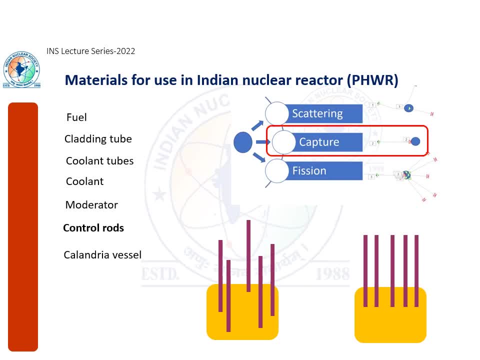 of neutrons is important for a material to be good control material. in the reactor there are two sets of control rods for two different functions: regulation and protection. one set of control rods adjust the power in the reactor core as per the requirement and this is called as. 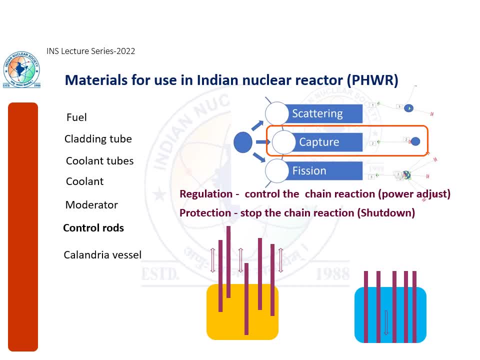 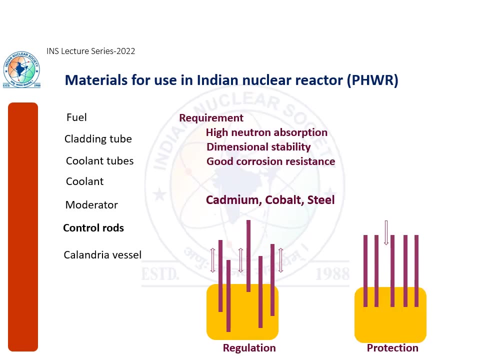 regulation. another set of control rods stops the fission chain reaction, resulting into shutdown of the reactor. when there is a trigger signal for stopping the reactor, this is called as the protection function. for the material to be a good control material, high neutron absorption capability is desirable. additionally, its dimensional stability and corrosion. 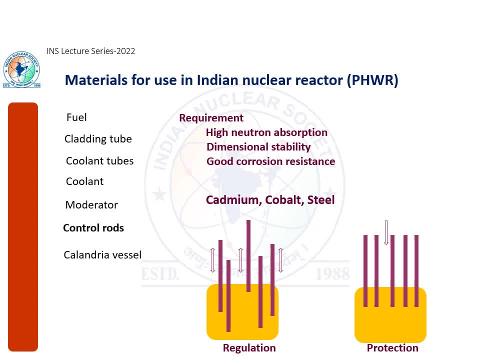 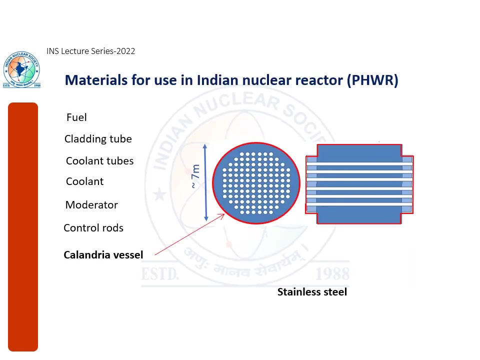 resistance become important for the desired performance. cadmium, cobalt, steel are the control rod materials that are used in PHWR, that is, pressurized heavy-water reactors. in India there are some designs that use boron also as control rod material. calendria whistle is the main component that. 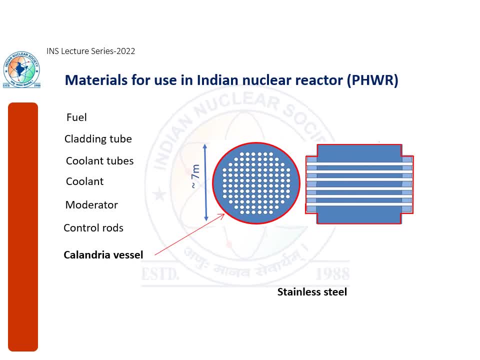 contains moderators. it supports coolant tubes with fuel bundles and also the coolant. it is a cylindrical horizontal structure. it is like enclosure and major support structure for reactor core components. it is typically made up of stainless steel material. here we can see a calendria whistle which is made up of stainless steel material. here we can see a calendria. 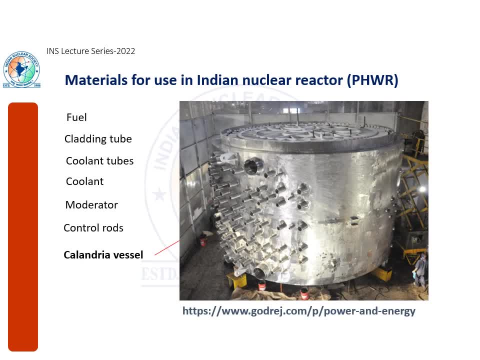 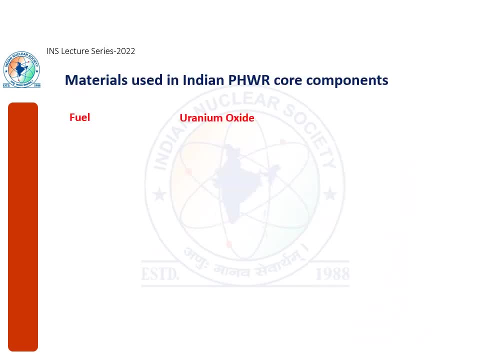 vessel for the latest PHWR as being manufactured by participation from Indian industries. so here we are summarizing all the different materials that are used in Indian PHWR, basically fuel coolant and moderator. they decide the type of the reactor cladding coolant tubes. they are made up of zirconium alloys. coolant & moderator are 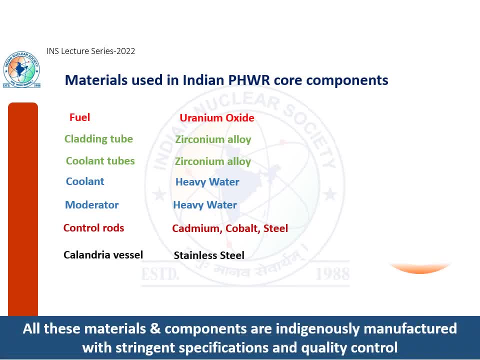 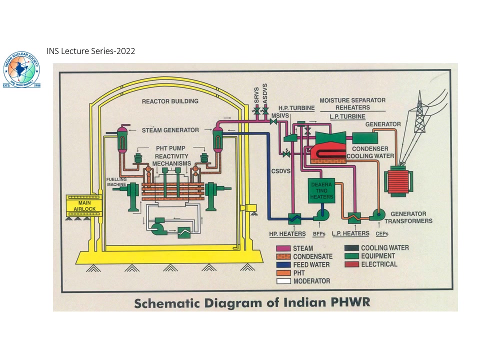 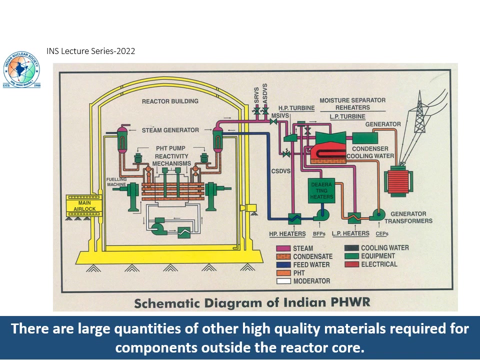 typically heavy water. these control rods are cadmium, cobalt and steel. the calendria vessel is made up of stainless steel. fuel in phwr is uranium dioxide, and all these materials and components are indigenously manufactured with stringent specifications and quality control. as we have seen, fuel coolant and moderator form the main components of reactor core and it governs. 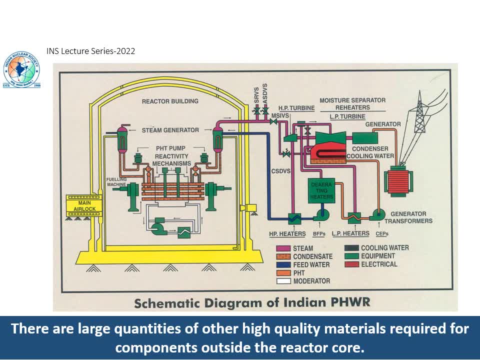 the type of reactor system. in addition to this, there are other non-core components which are outside the reactor core but important for safety and other functioning. some of these materials have functional requirements for shielding, fuel handling, steam generation, cooling and circulation, etc. some of these materials have stringent requirements because they cannot be. 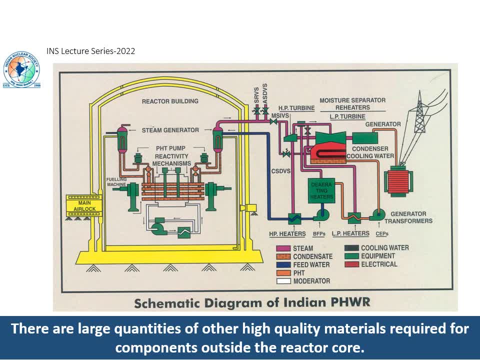 accessed after the reactor starts operation, or due to layout considerations or due to reactivity or radioactivity, or may be physical barrier. so in general there are large quantities of other high quality or nuclear grade materials that are required for non-core components also within the reactor building material. technology development is not as easy as it. 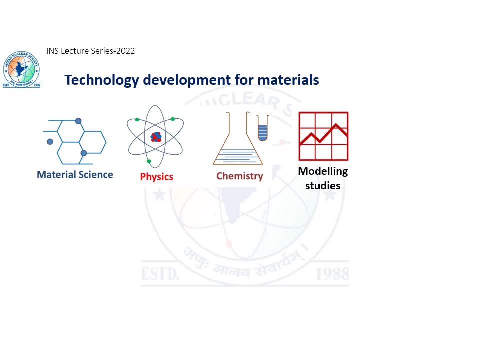 appears. we need to understand the material science, its metallurgy, crystal structure, the physics and the chemistry aspects that govern the material behavior. the destructive and non-destructive testing is very essential for evaluation of mechanical, chemical, thermal or metallurgical properties. it should be possible to manufacture the component from the material to achieve the 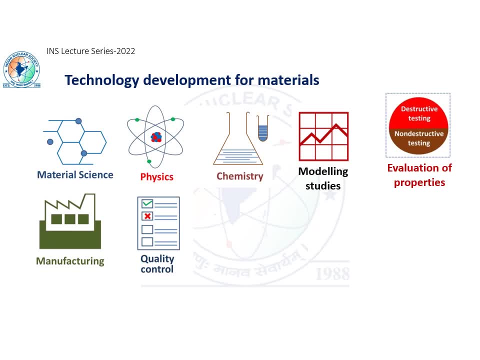 desired complex geometry product with unique properties for the intended function. the component design has to be assessed thoroughly by analysis as well as by experiments under radiation environment to establish confidence about its performance. this is done in research reactor for studying the material irradiation behavior. all these help in finalizing the technical specifications. 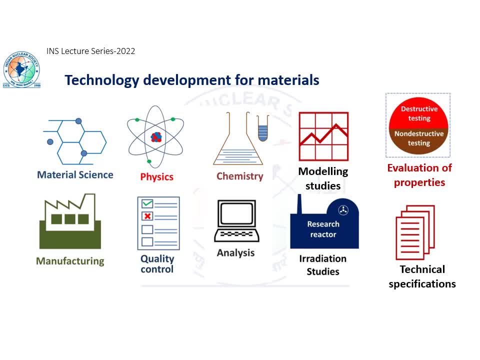 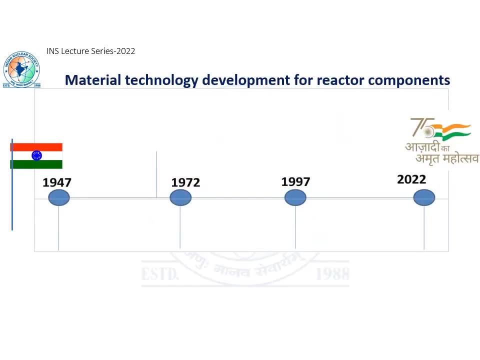 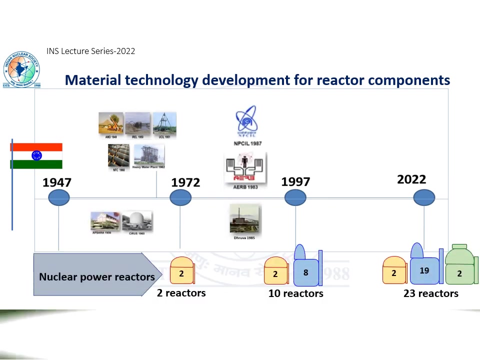 for each of the different components for reactor core. thus, we see that the expertise from various domains of science and engineering is necessary to develop special materials for reactor core components. india got independence in 1947 and this year, in 2022, we are celebrating 75 years of independence. that is azadika amrut mathso. 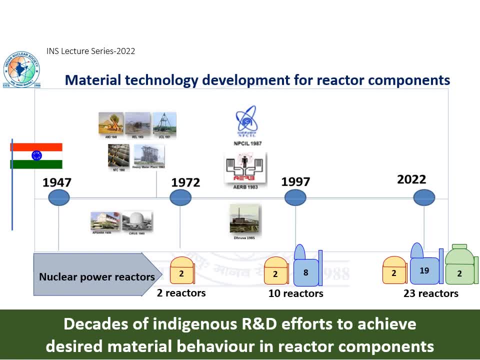 in terms of number of reactors, there were two nuclear power reactors and two research reactors operating after 25 years of independence. additionally, all the necessary facilities and plants were built and made operational for exploration, mining and processing of nuclear fuel- material uranium, and then manufacturing of fuel bundles for use in reactors. 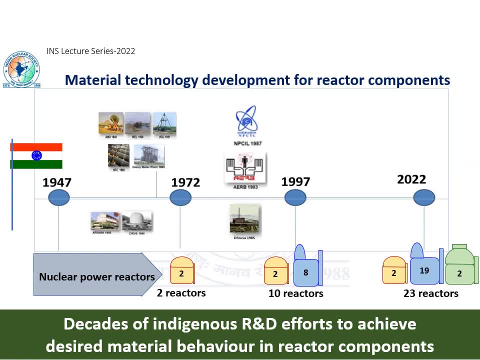 as the need was felt, npcil nuclear power corporation was formed to take care of operation and maintenance of growing number of nuclear power plants in india. similarly, a regulatory body- atomic energy regulatory board, aerb- was created for review, monitoring and regulation of various nuclear special facilities in country. number of 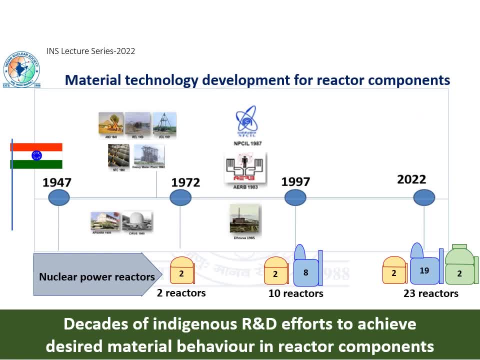 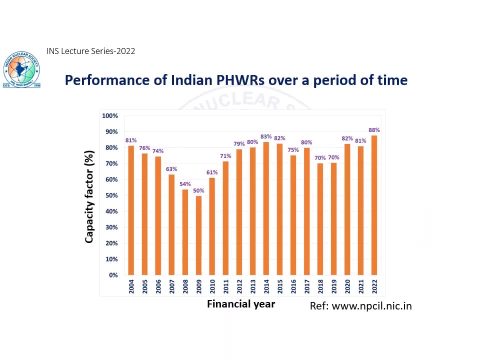 reactors have doubled and installed electrical capacity has tripled in last 25 years. thus decades of indigenous r&d efforts have helped to achieve the desired material behavior in reactor components. this shows the capacity factors for the last almost uh 17 to 18 years of indian pressurized 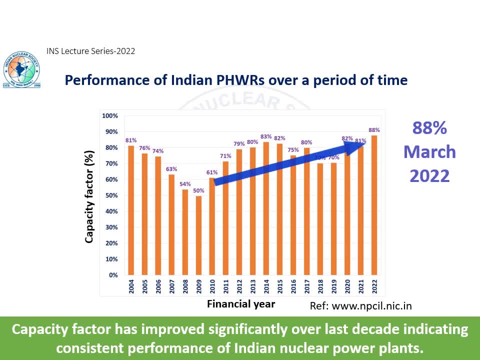 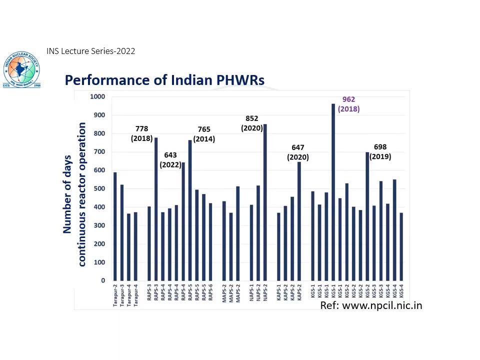 heavy water reactors. As we can see from here, the capacity factor has increased from 60% to 88% over the last about 12 years. This is significant improvement, indicating consistent performance of Indian nuclear plants. Here we have plotted the number of days of continuous operation for different nuclear power plants in India. 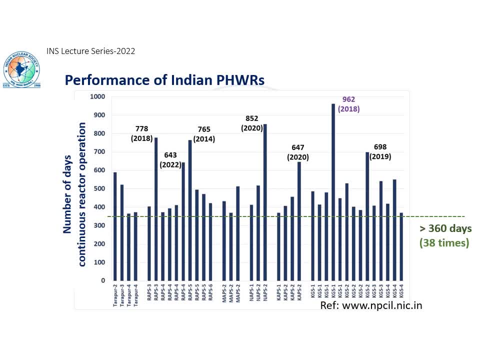 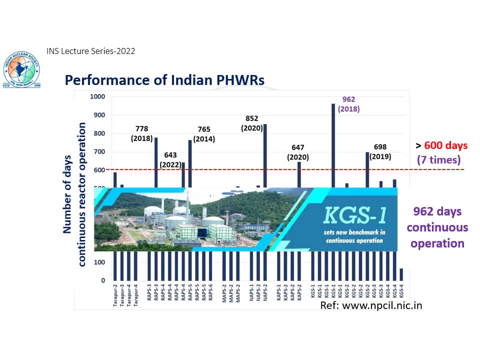 As we can see, there has been continuous operation of more than 360 days at more than 38 occasions. Also, more than 7 times the plants have operated for 600 days plus duration. Kaiga Unit 1, located in the northern Karnataka, has operated for continuous 962 days of operation in the year 2018.. 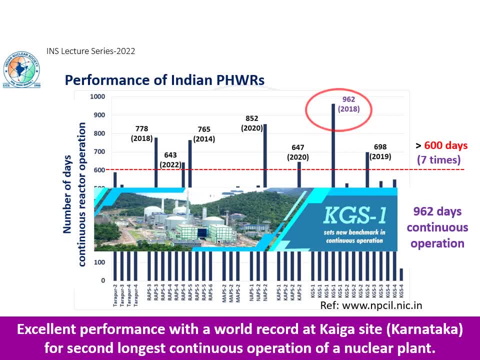 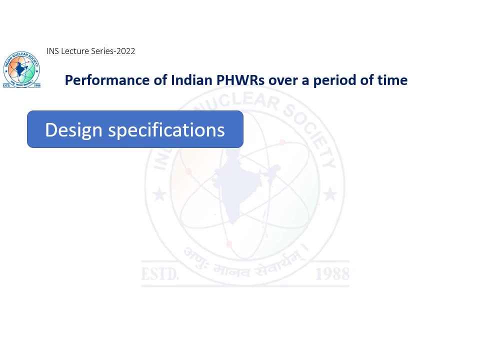 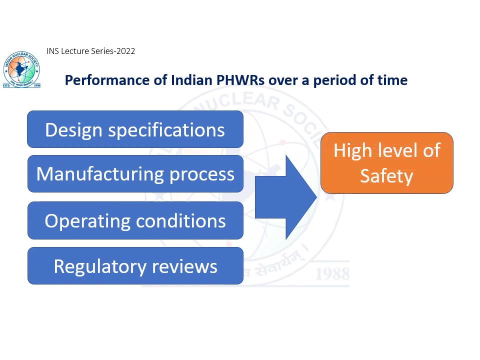 Excellent performance with a world record. This is the report at Kaiga site for the second longest continuous operation of a nuclear plant: Design specifications as per international standards, manufacturing processes with strict quality control, operating conditions and parameters of reactor core, along with the periodic rigorous reviews by regulatory body.